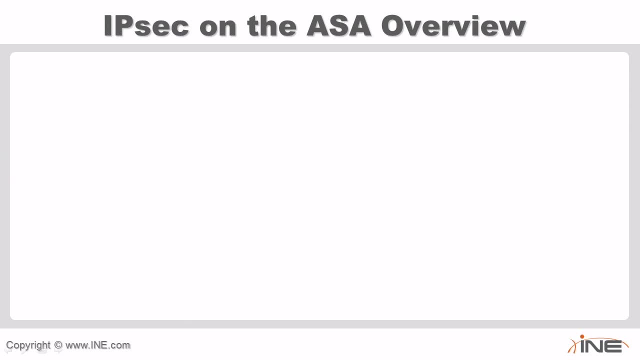 configuration syntax and the configuration logic of IPSec on the ASA is going to be a mix between the iOS and the previous VPN 3000 concentrator that the ASA got a lot of its underlying logic for with the tunnel groups and with the group policies. Now we'll see that, like the iOS, 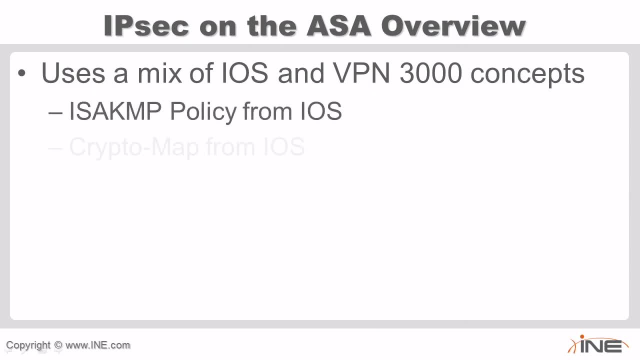 the ASA still does use ISA camp policies and it does use crypto maps, which are going to be used to define our phase one and phase two parameters for the majority of IPSec options. Then we'll have the tunnel groups and the group policies that came from the VPN concentrator that are going to 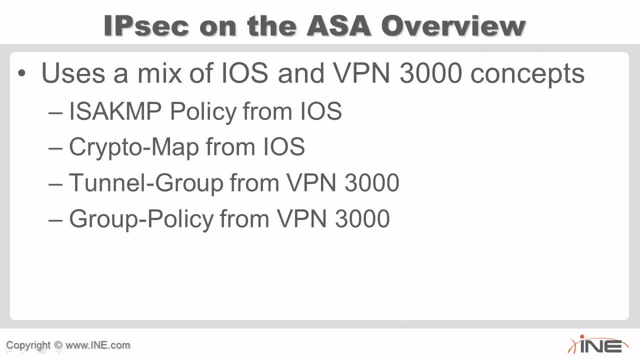 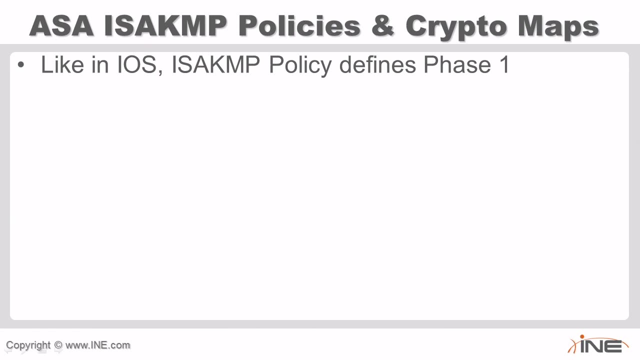 be used to apply the tunnel groups and the group policies that came from the VPN concentrator. Now we're going to define our phase one parameters with the ISA camp policy, which is going to be things like the authentication, the hash- whether we're using MD5 or SHA- is the encryption single. 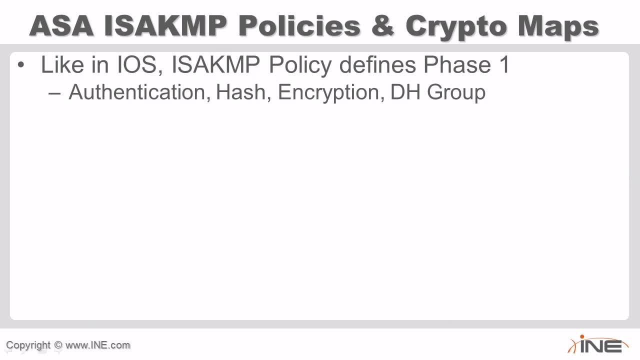 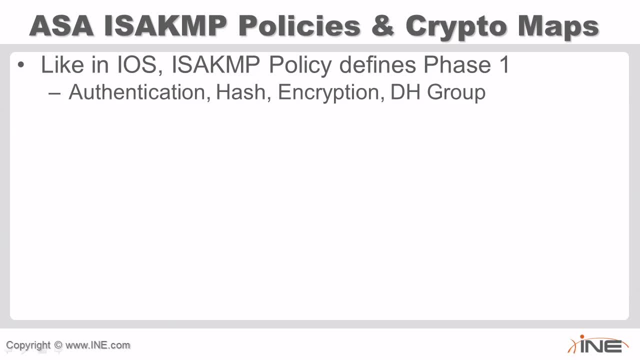 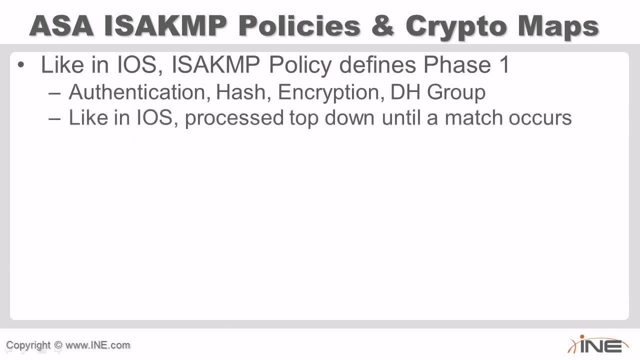 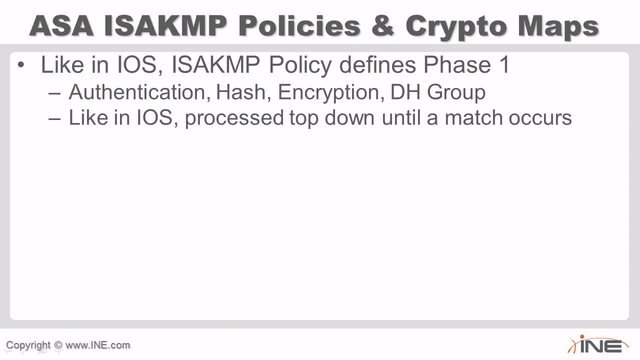 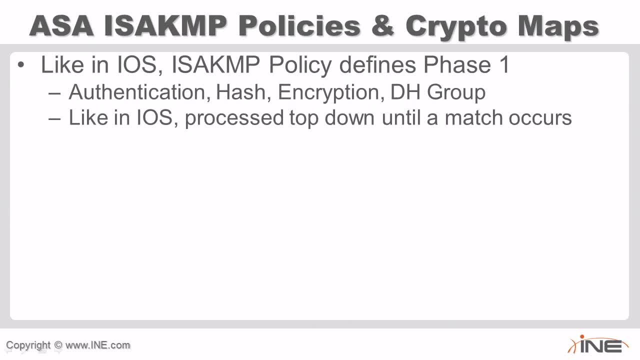 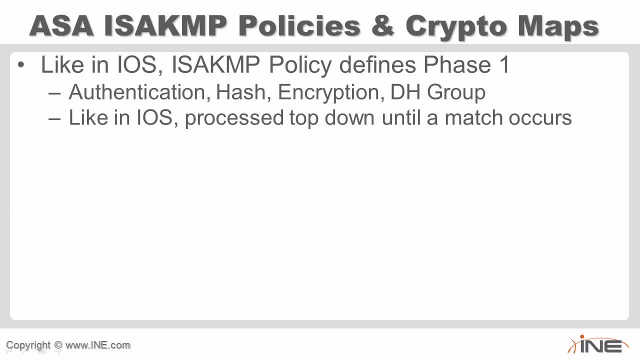 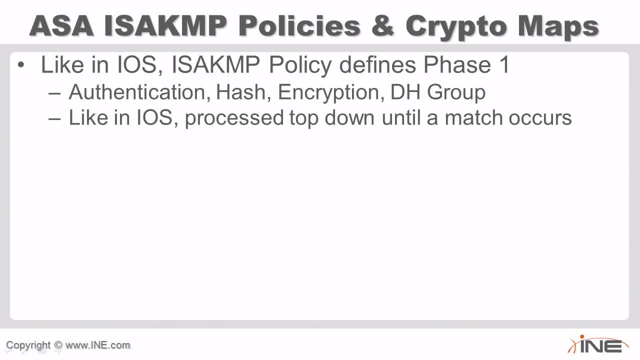 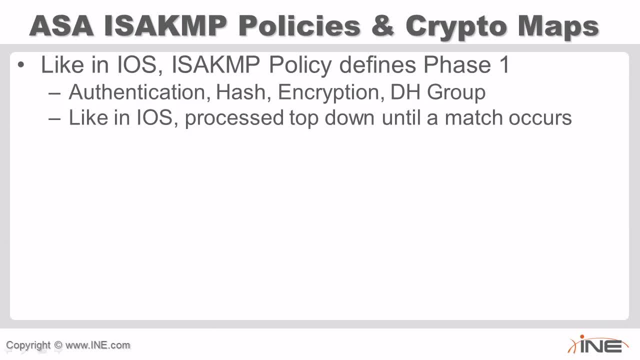 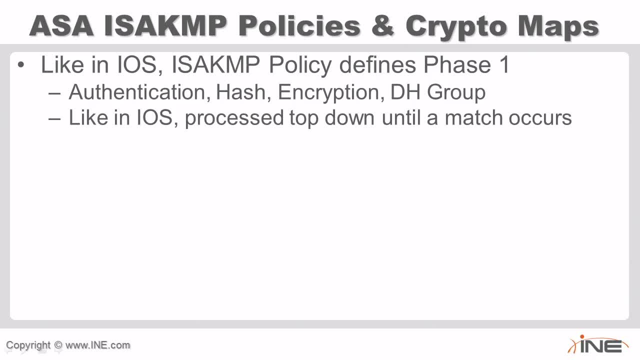 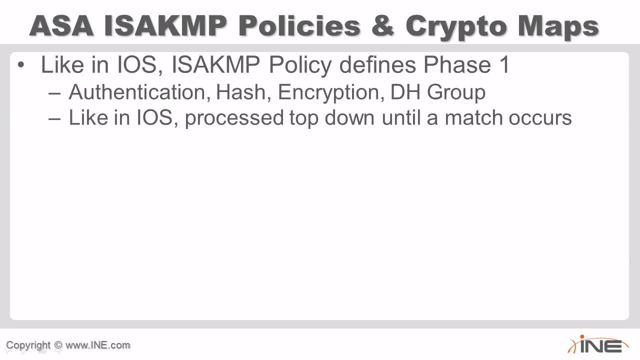 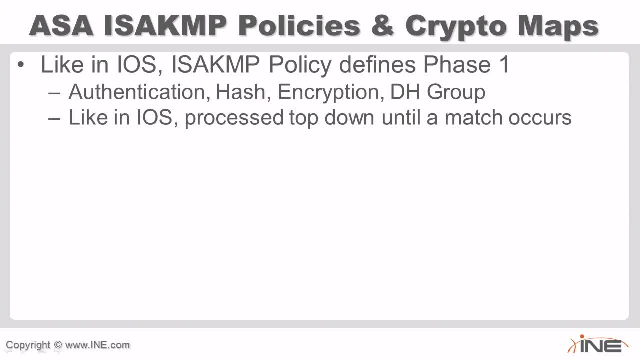 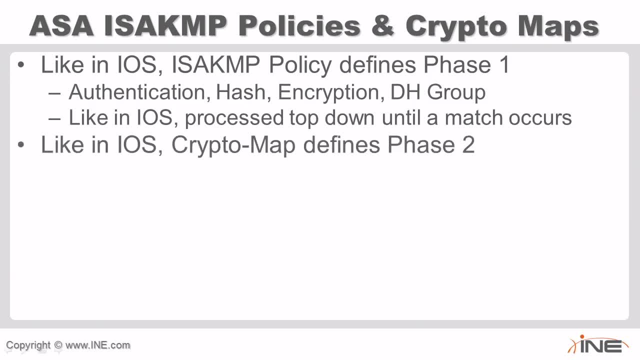 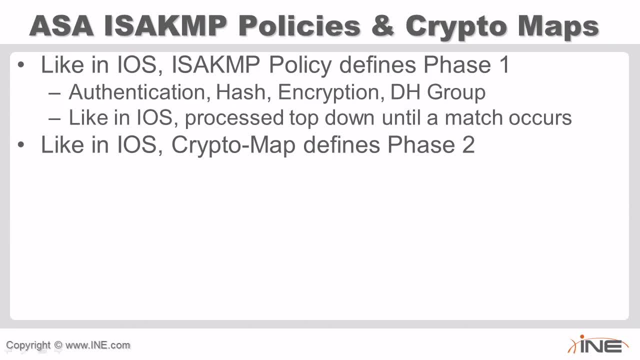 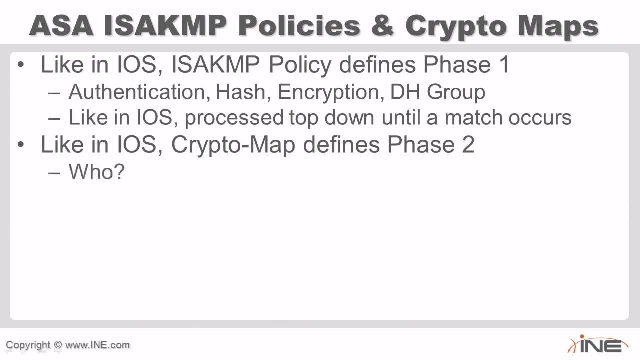 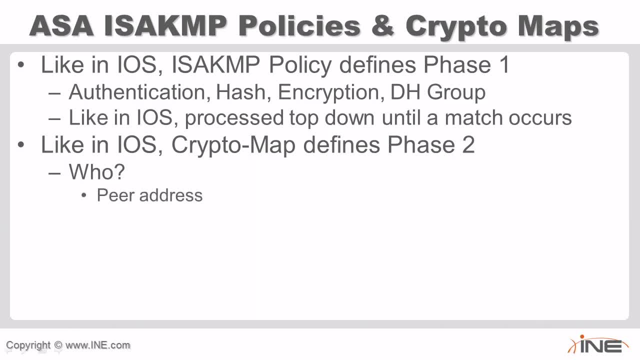 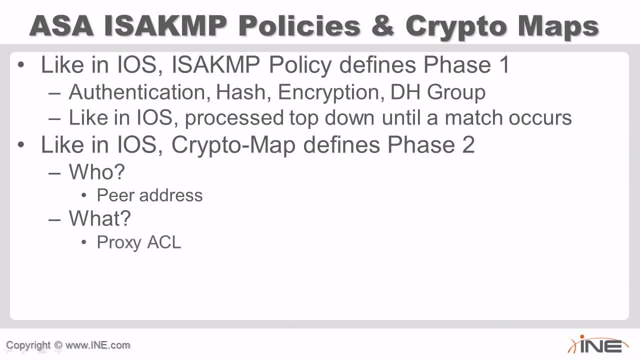 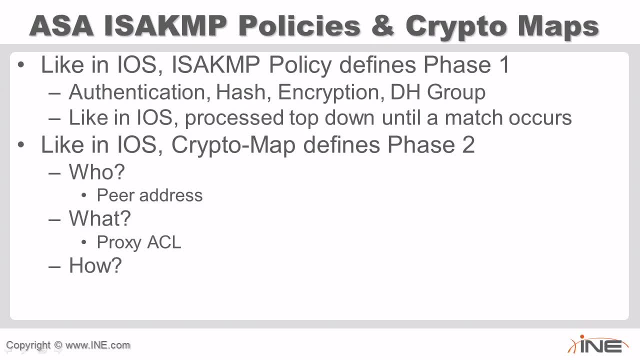 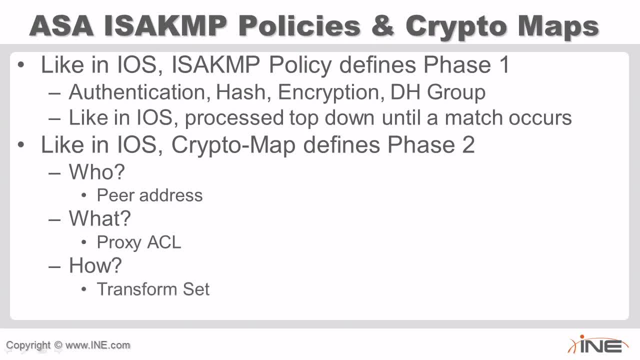 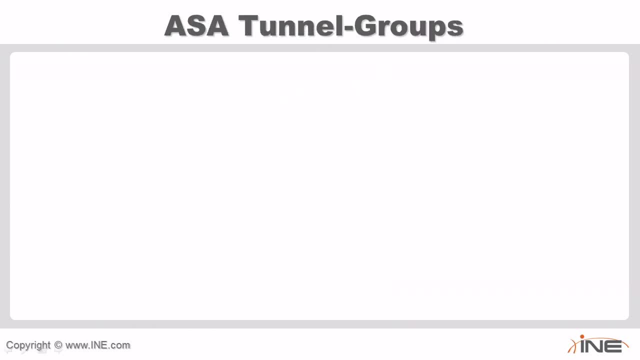 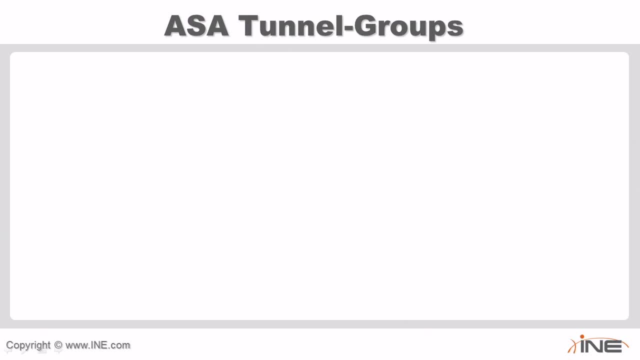 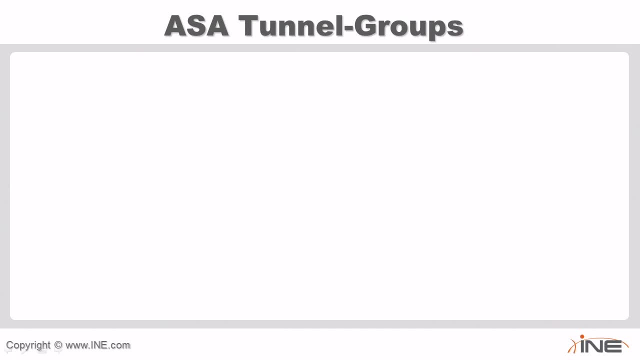 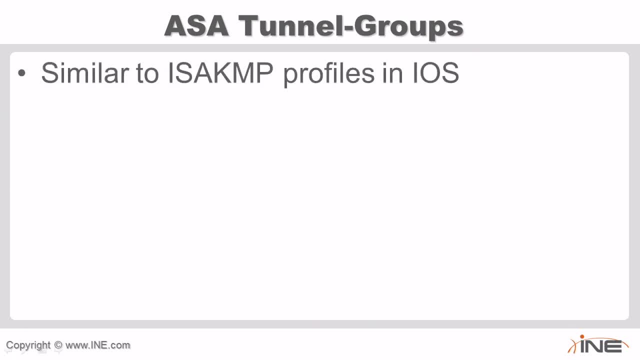 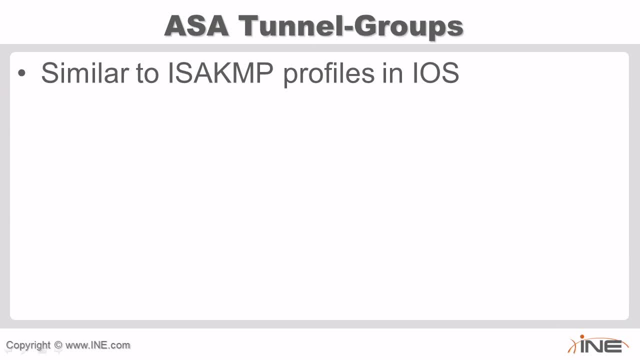 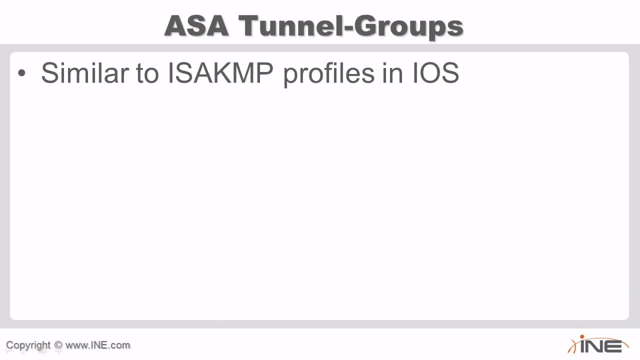 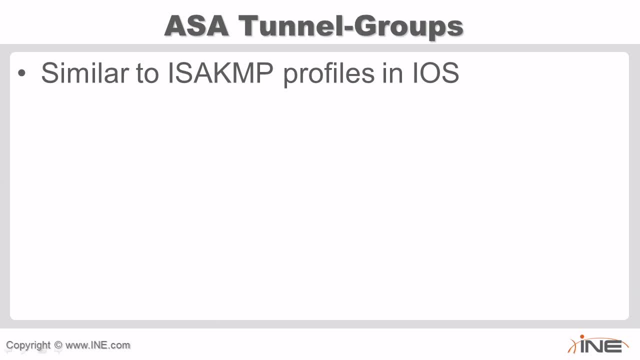 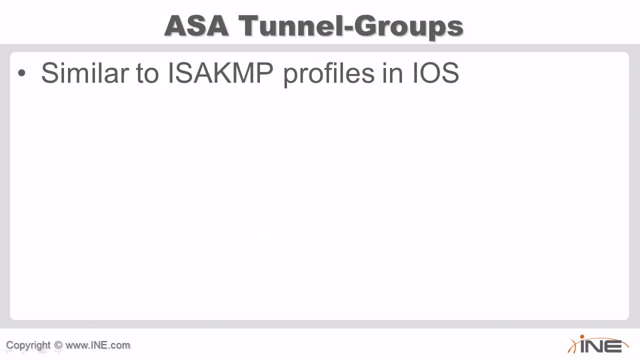 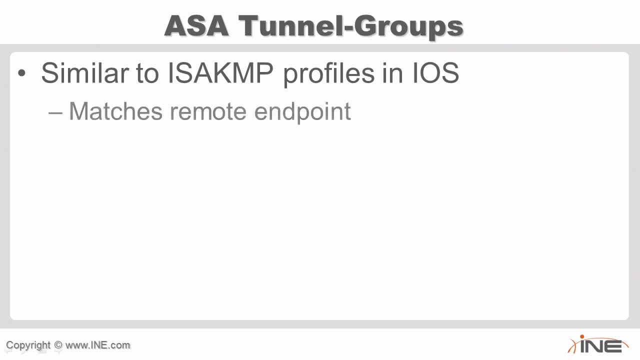 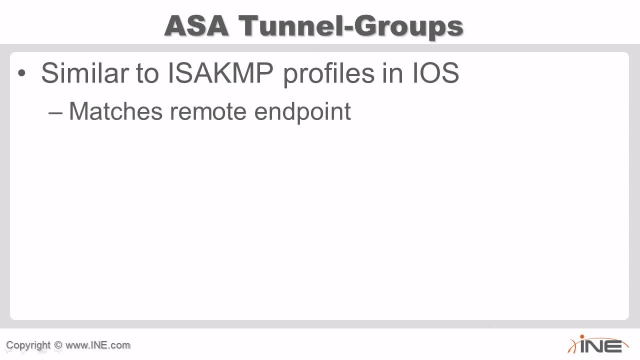 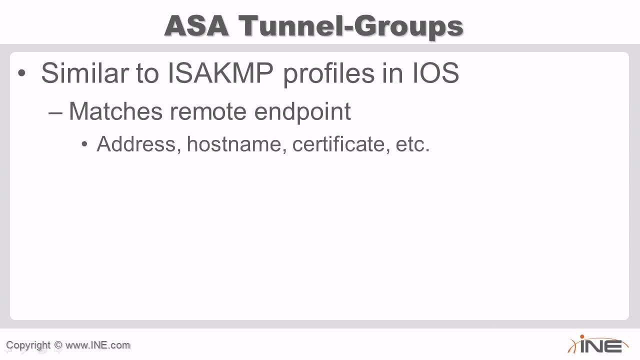 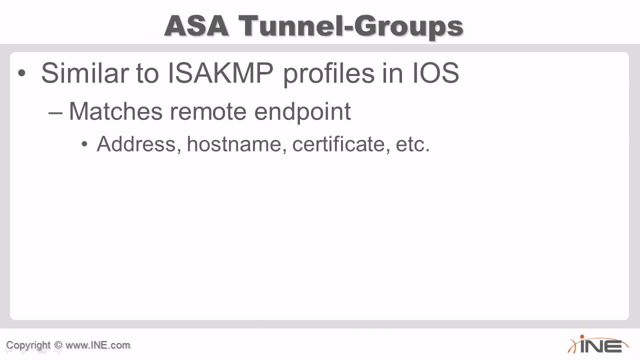 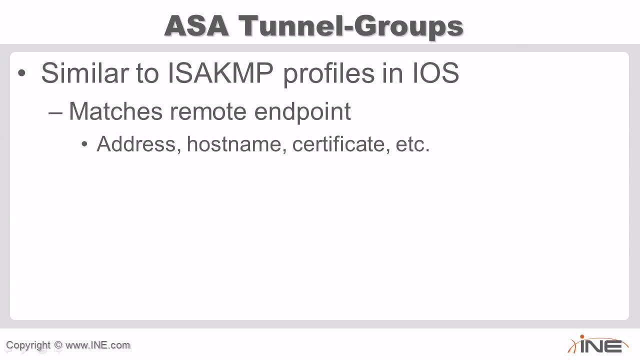 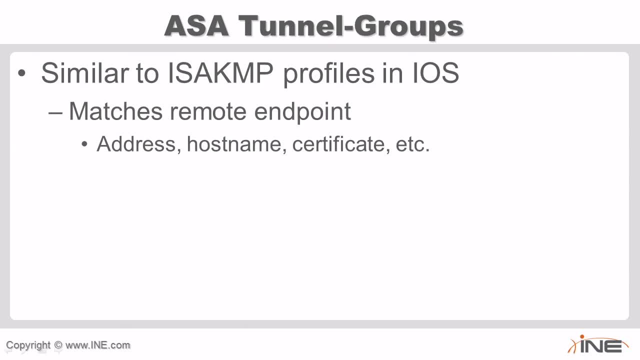 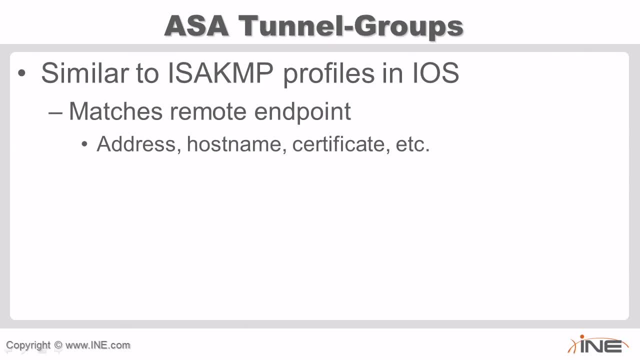 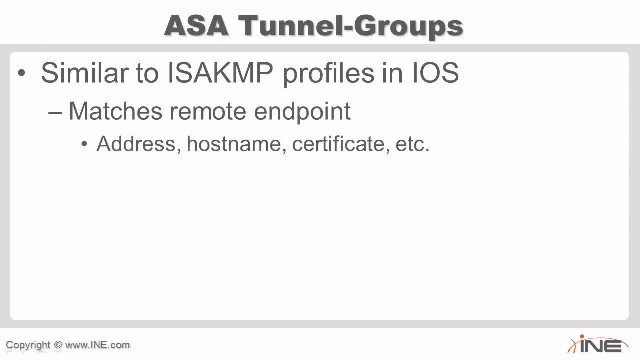 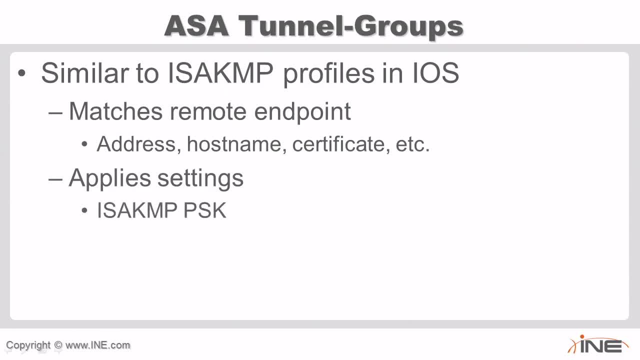 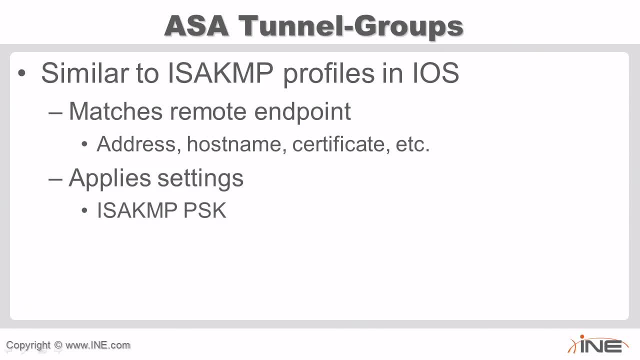 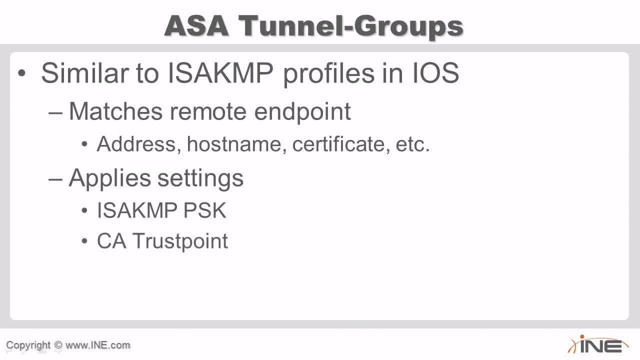 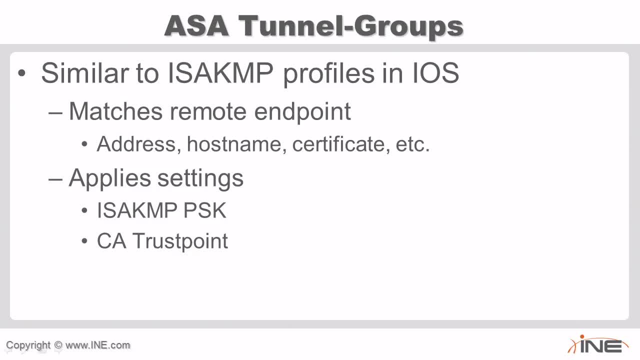 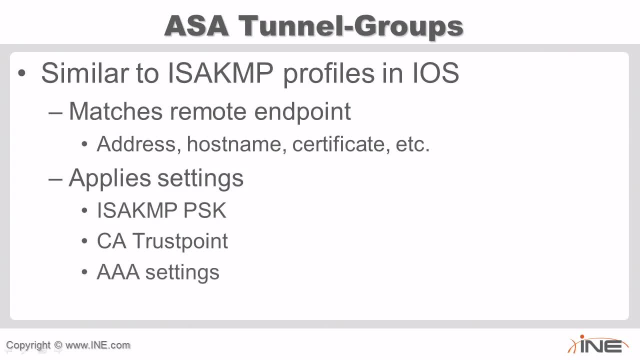 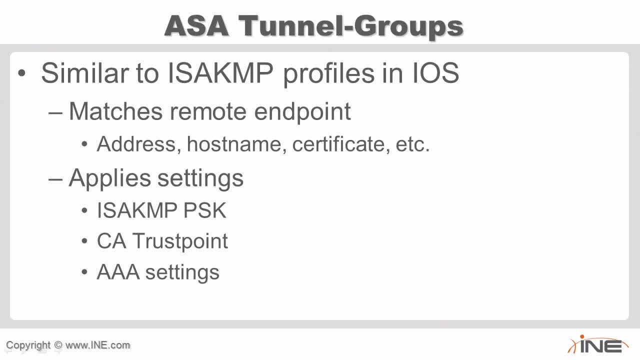 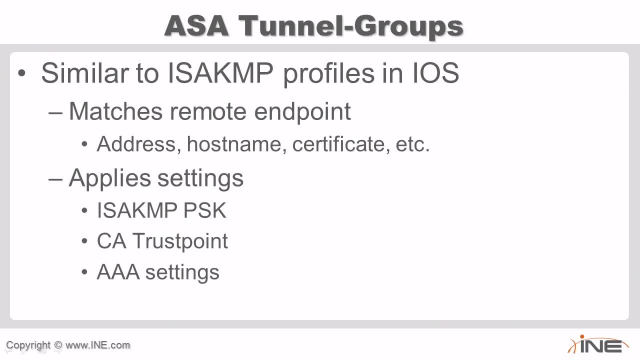 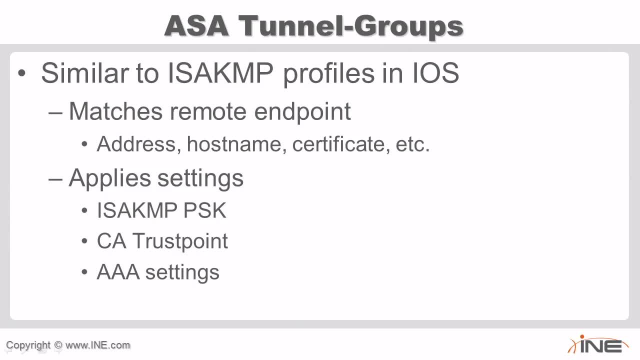 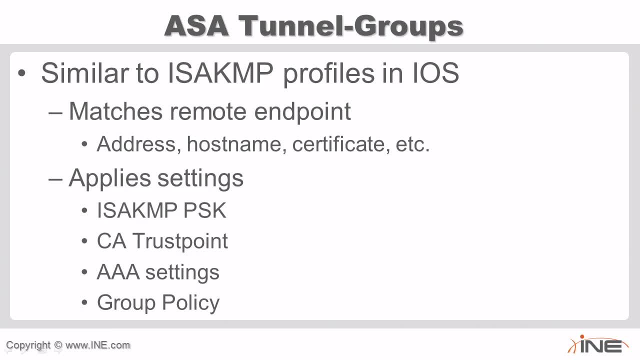 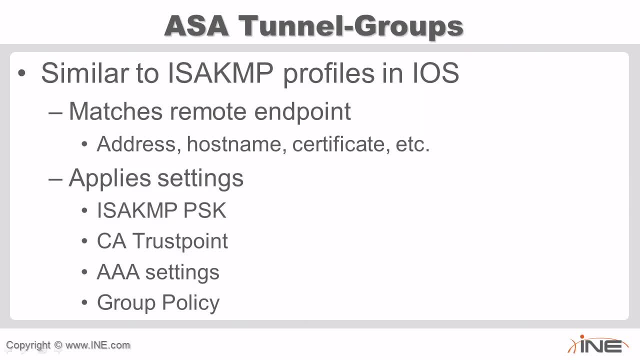 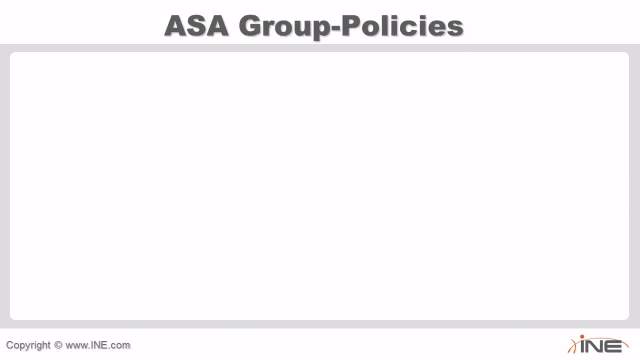 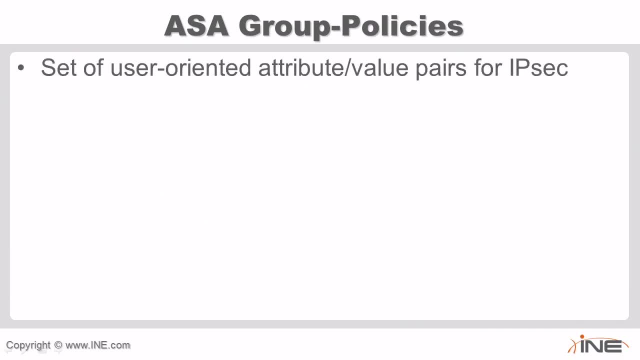 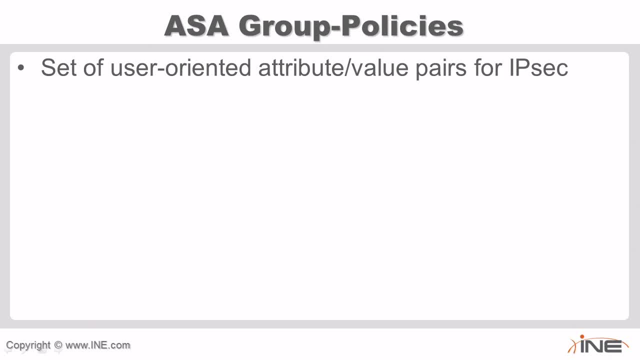 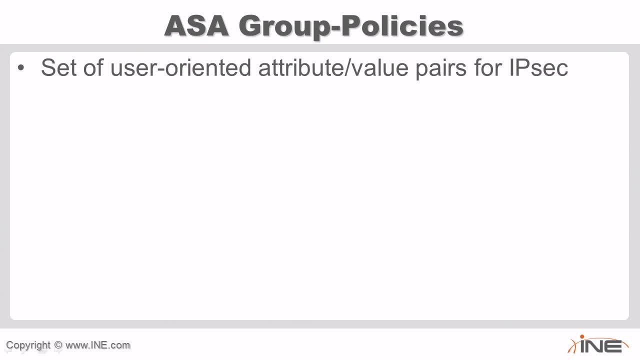 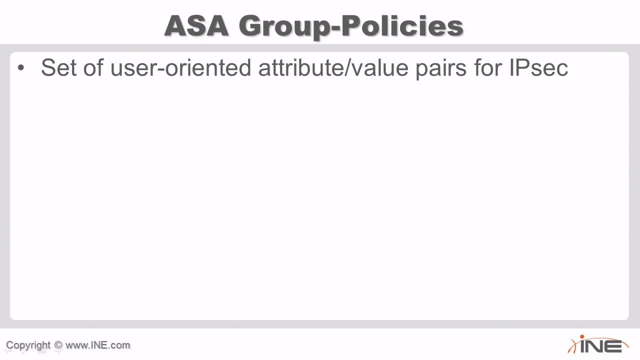 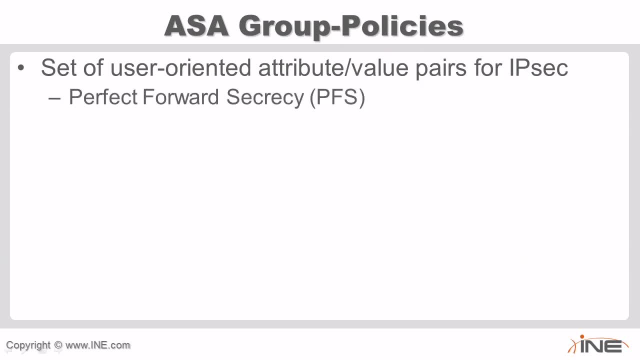 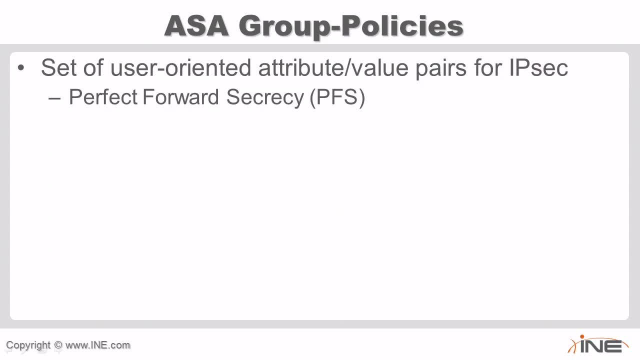 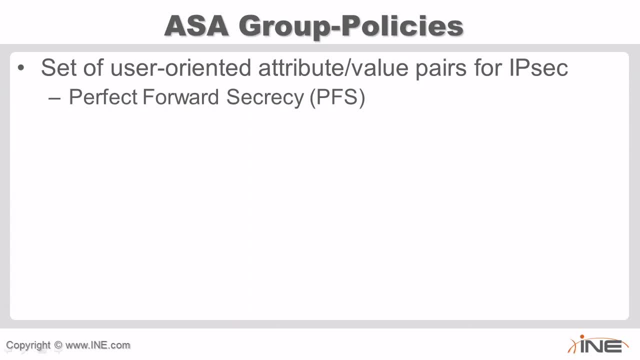 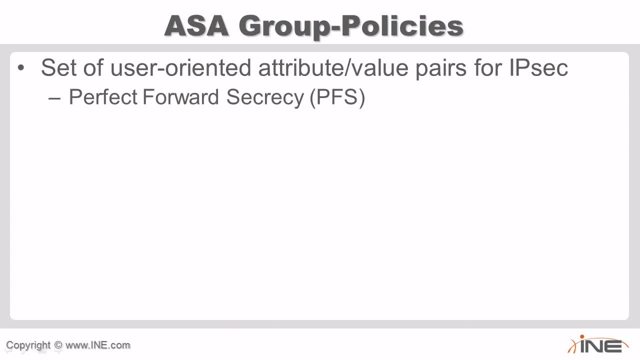 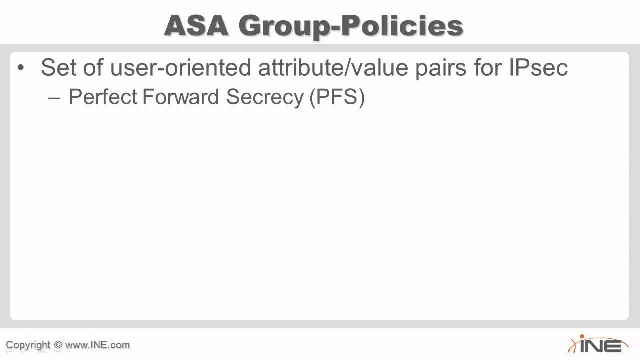 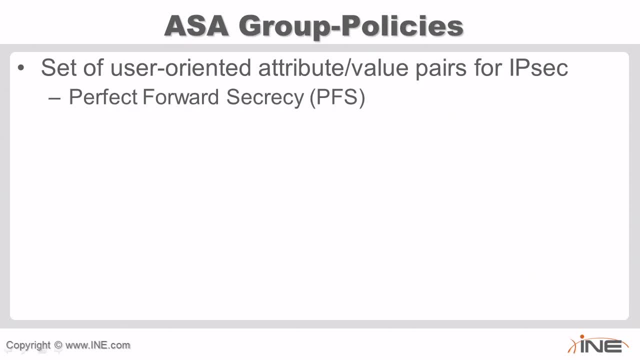 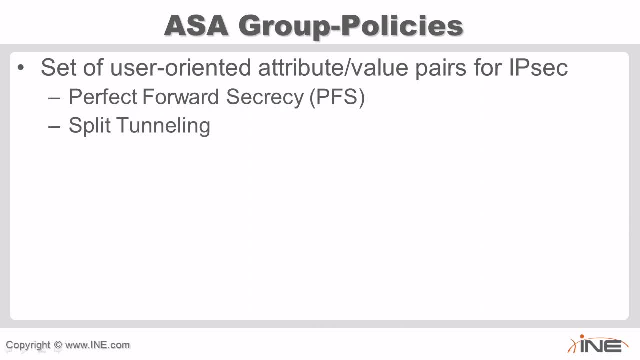 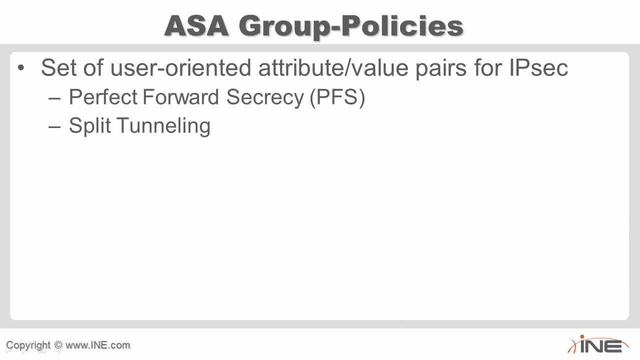 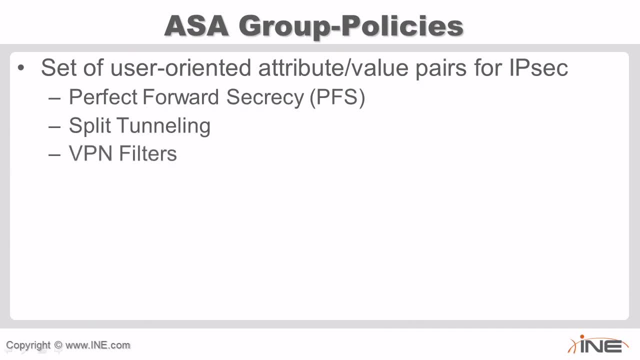 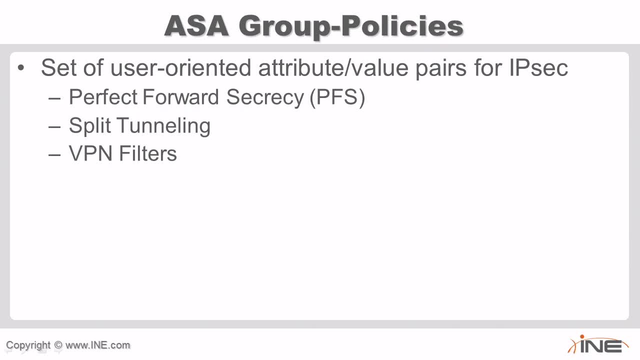 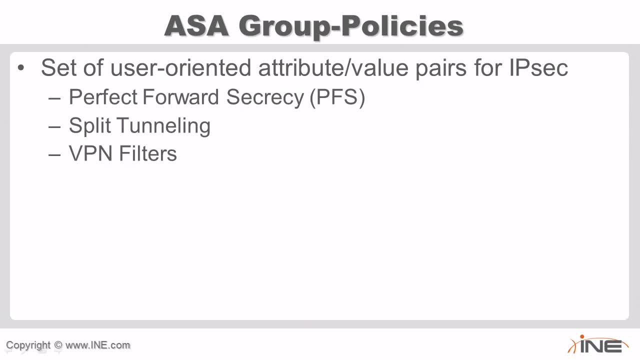 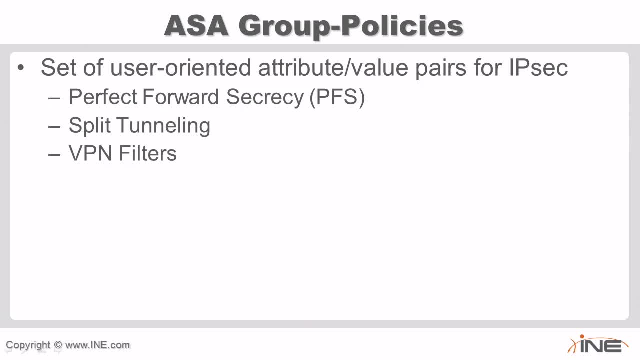 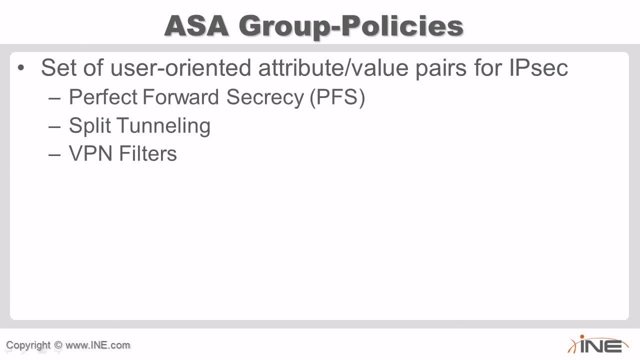 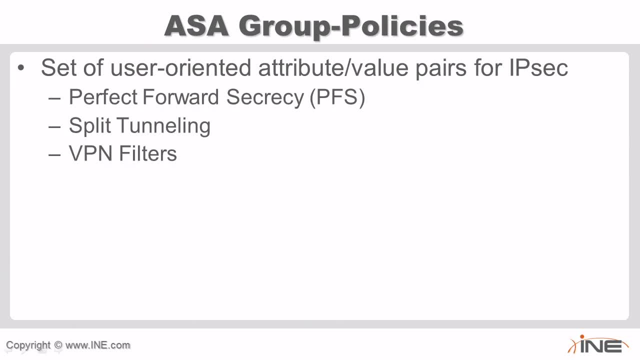 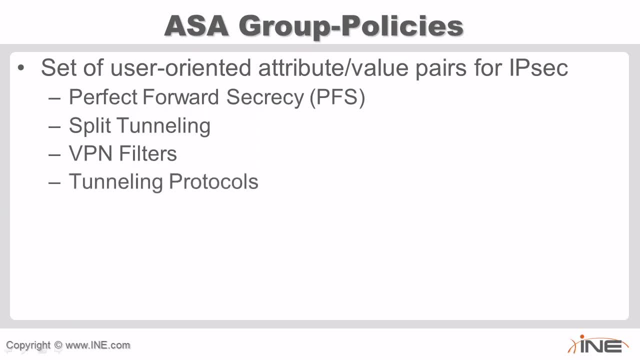 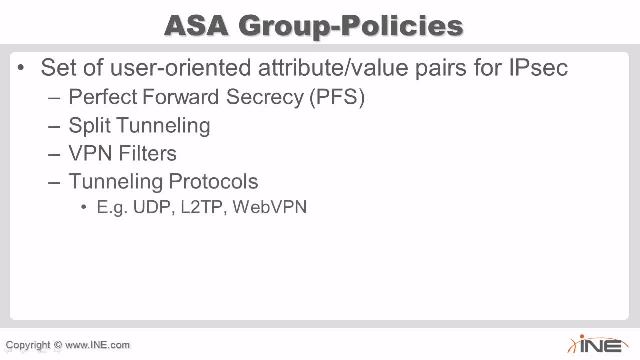 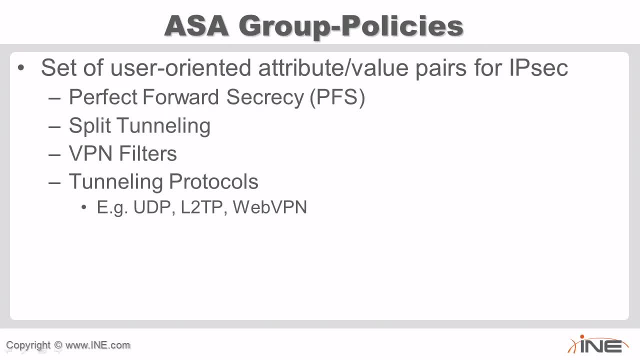 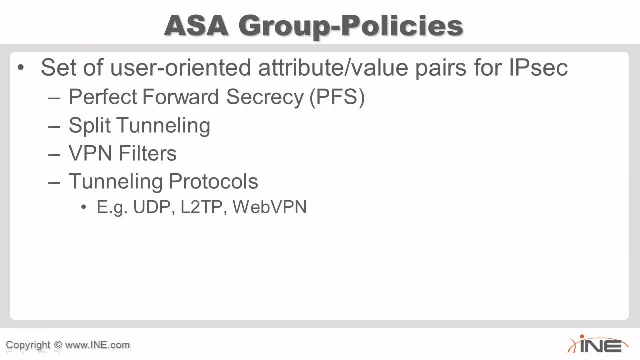 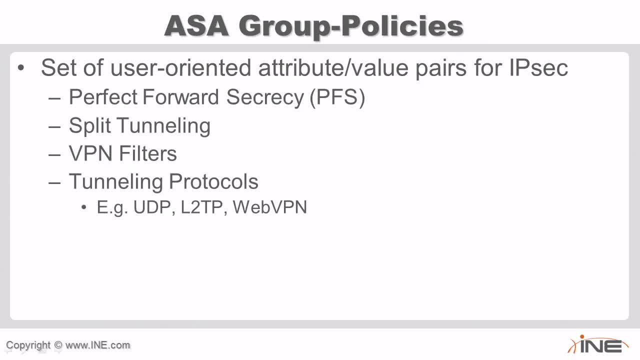 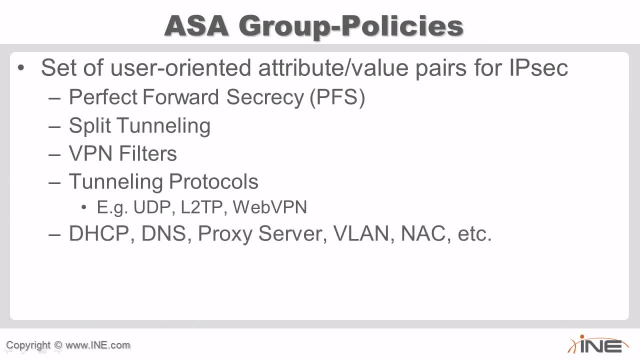 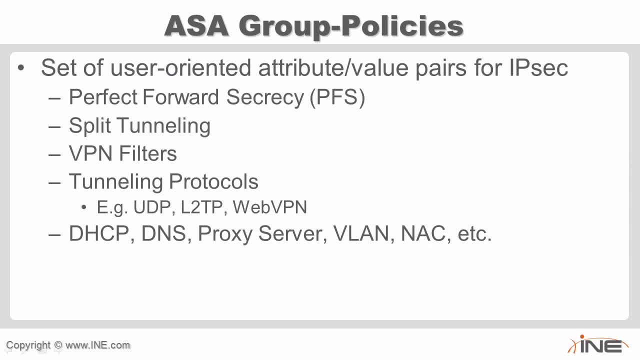 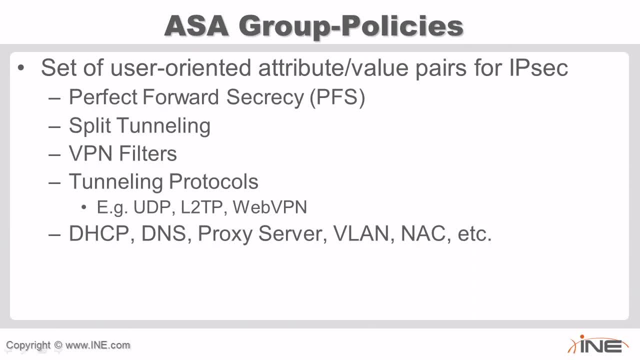 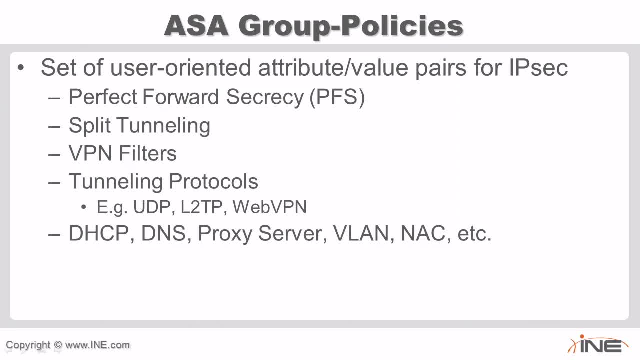 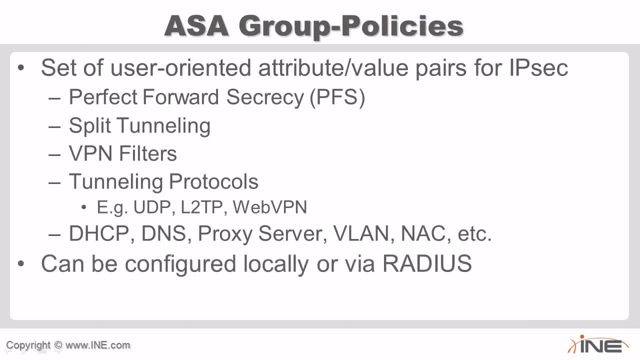 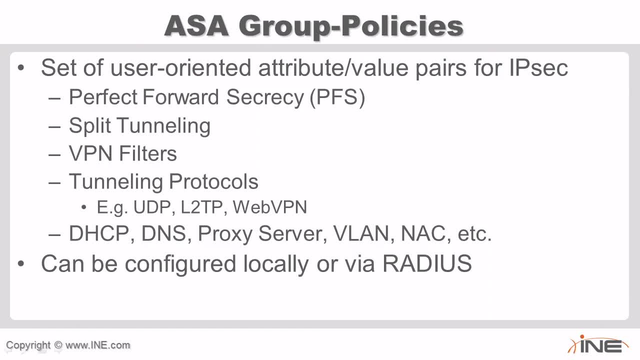 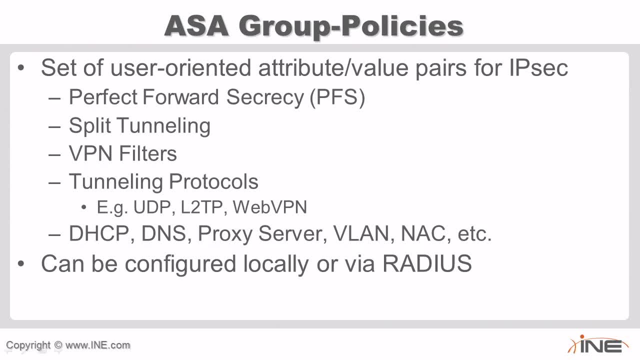 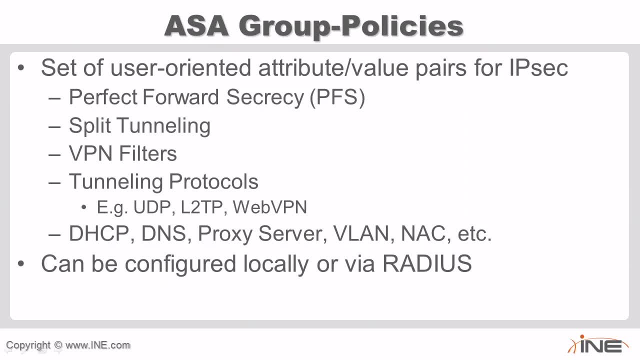 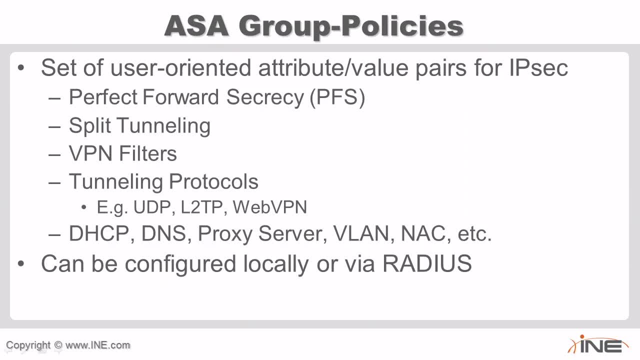 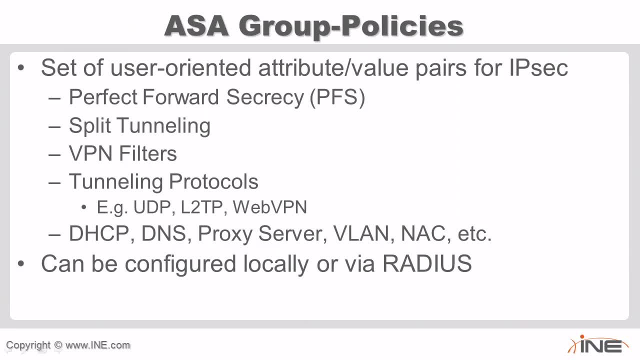 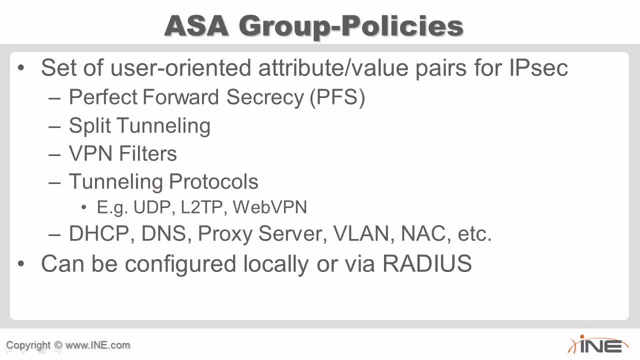 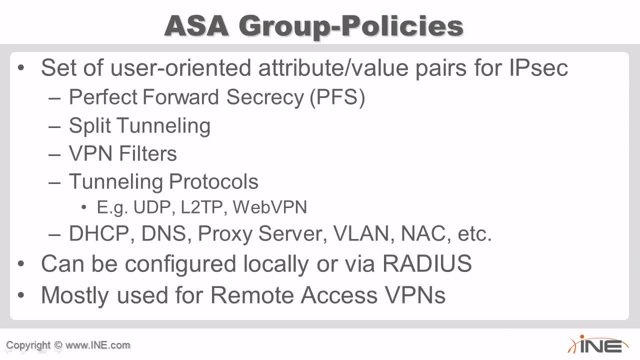 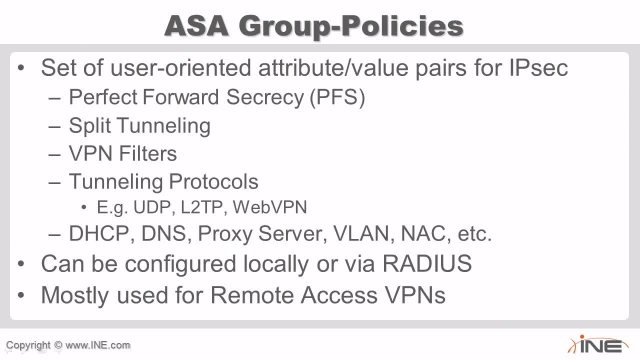 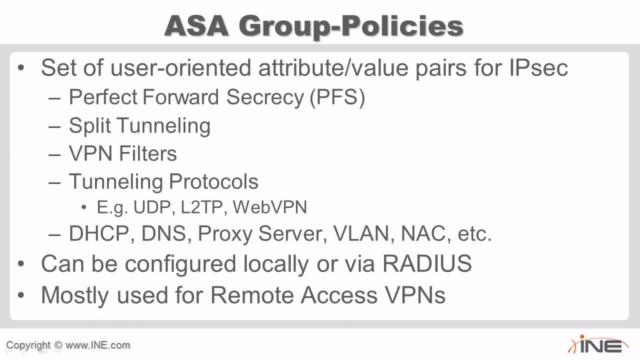 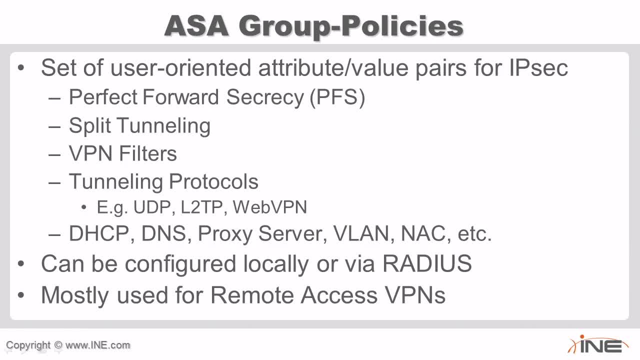 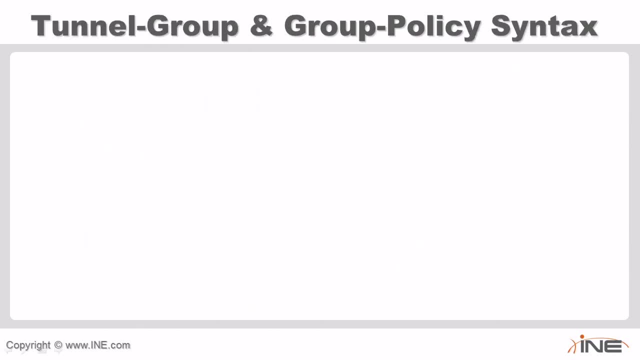 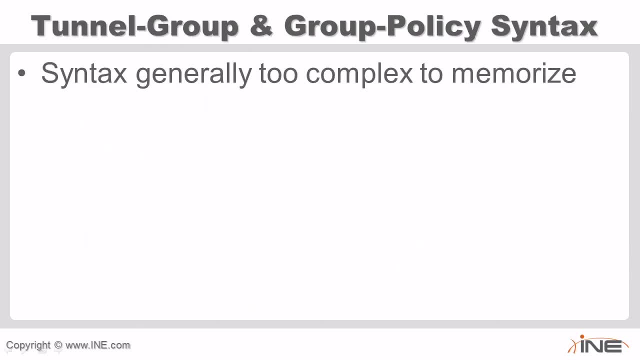 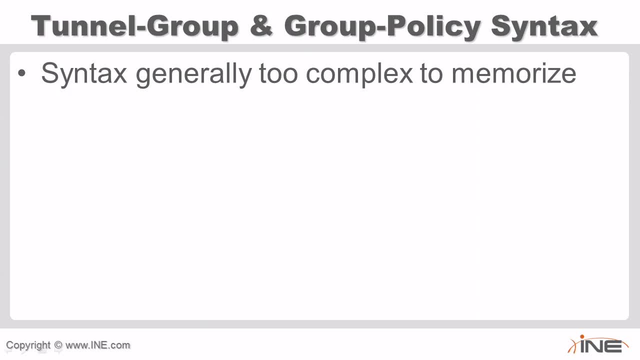 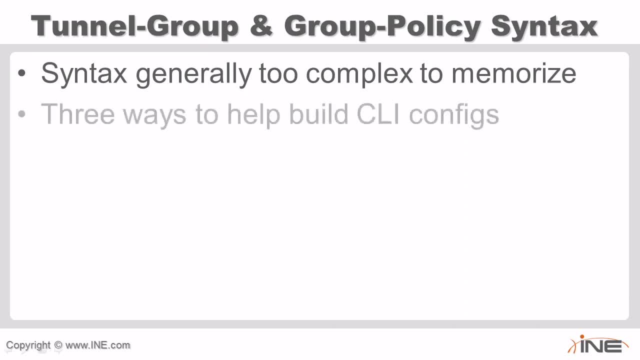 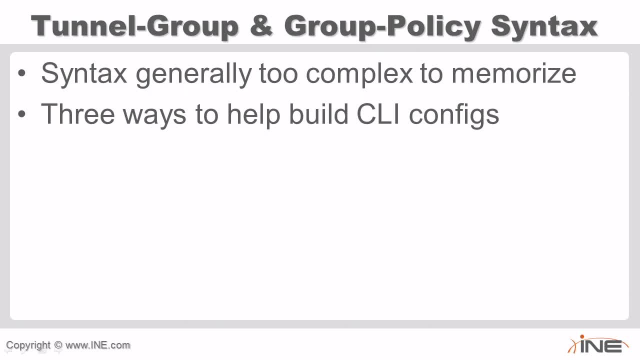 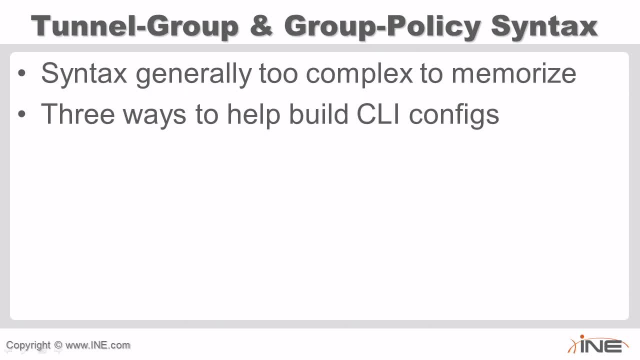 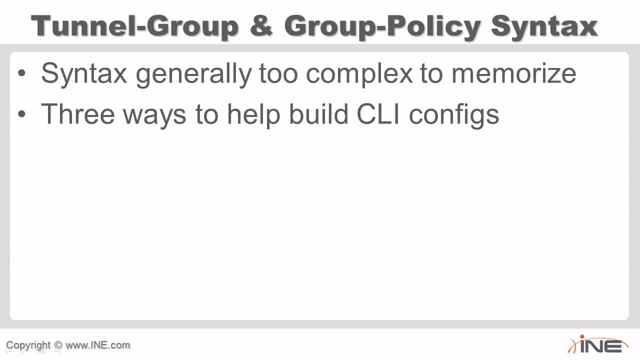 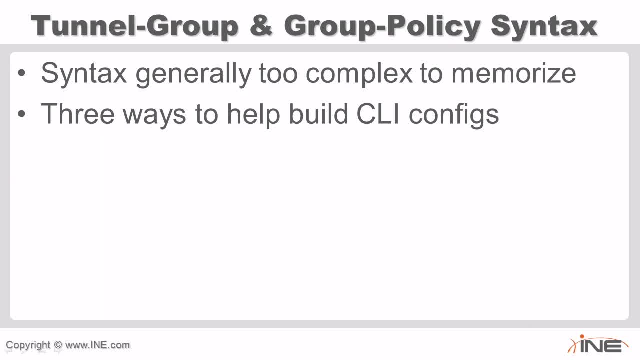 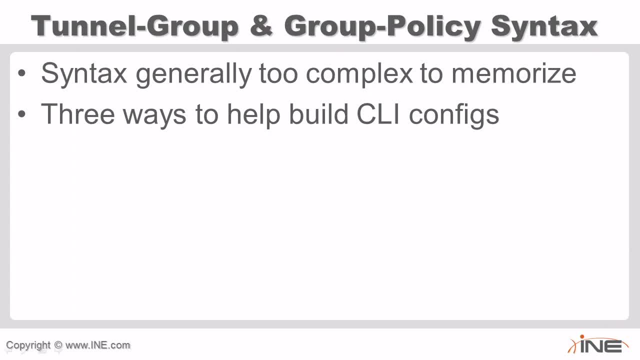 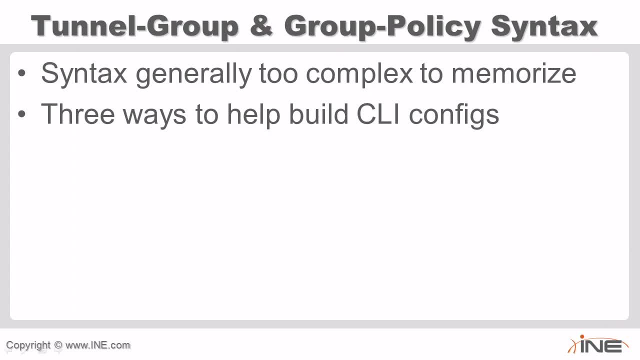 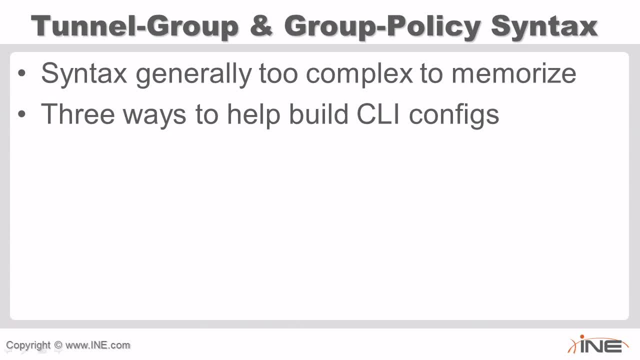 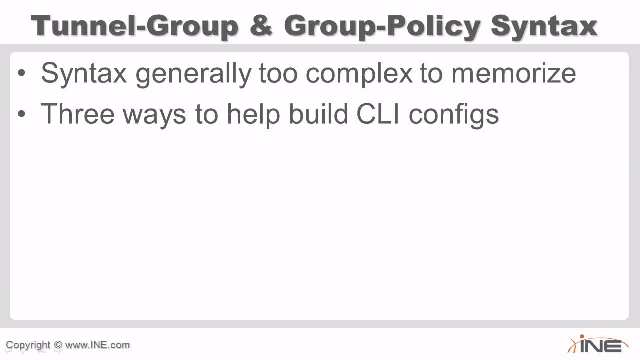 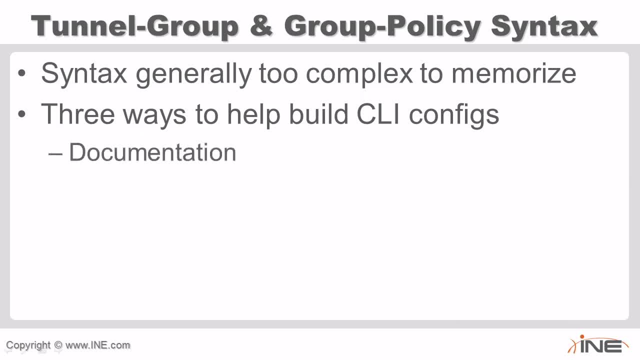 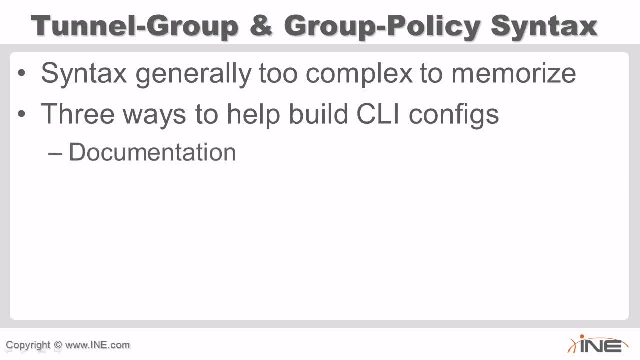 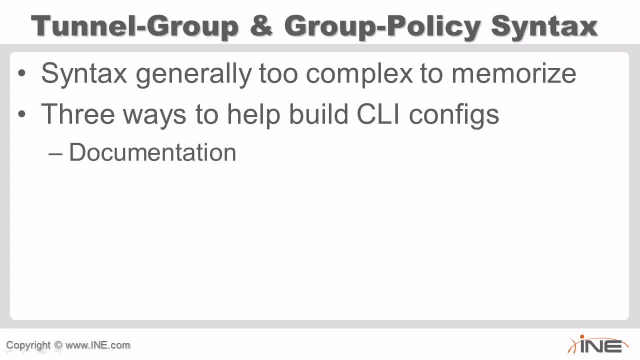 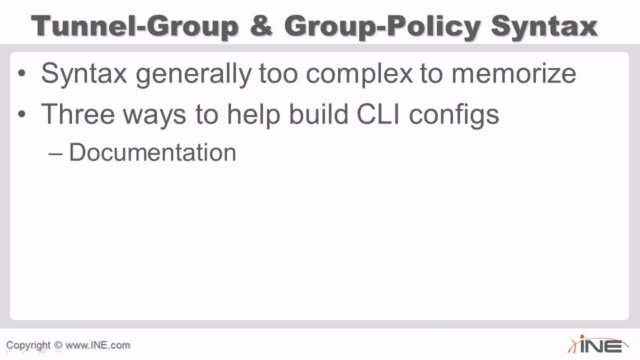 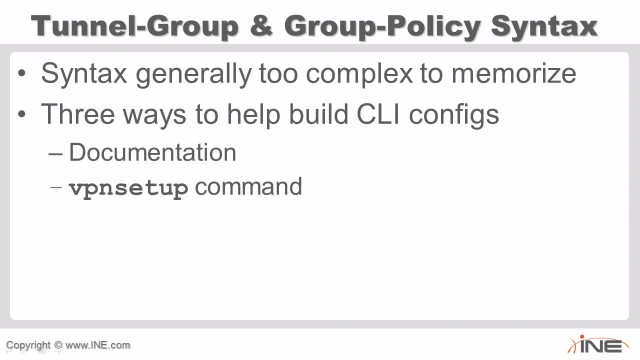 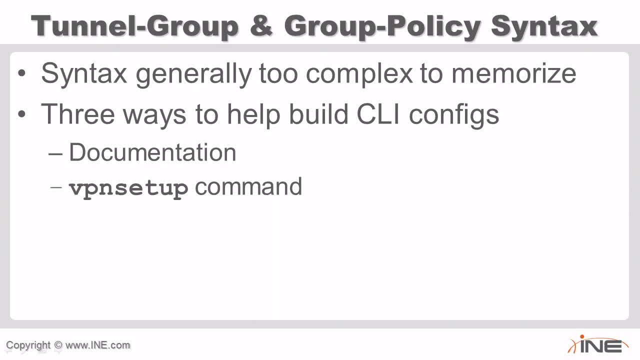 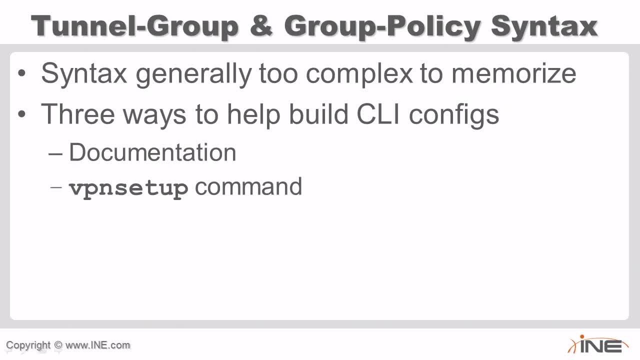 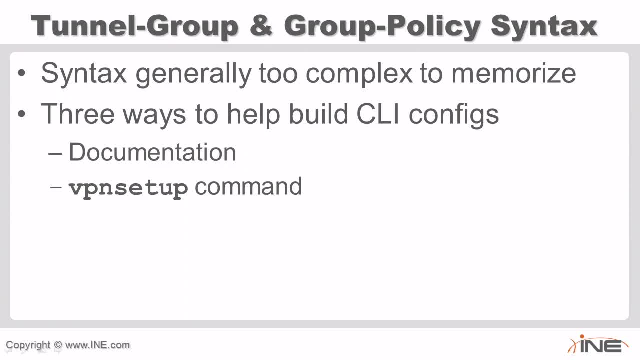 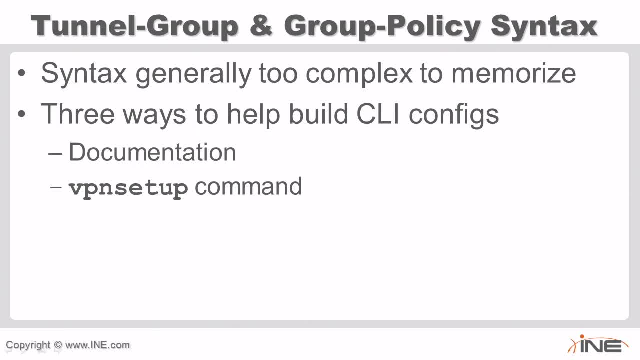 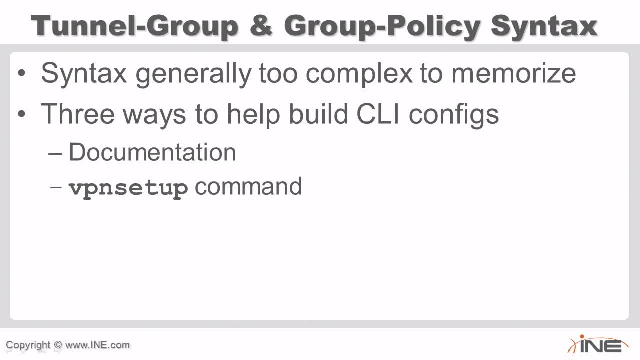 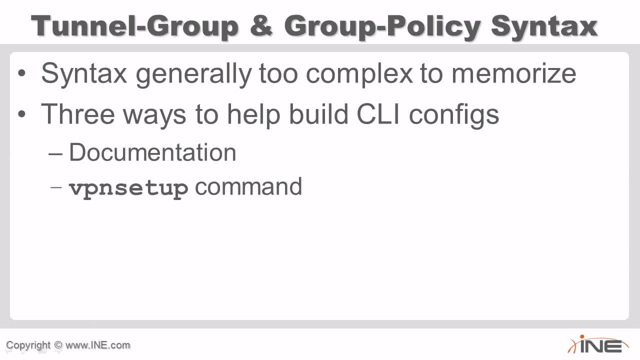 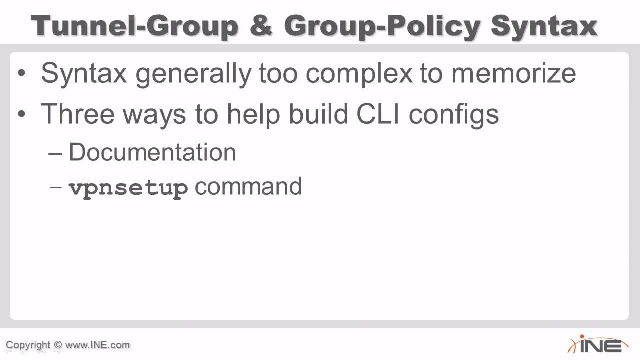 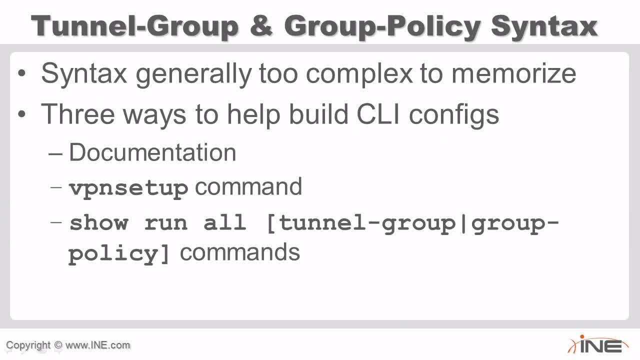 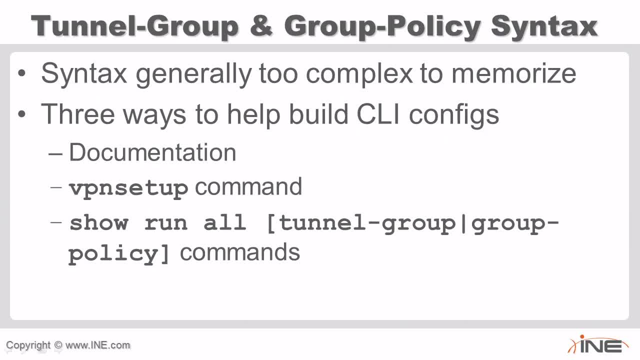 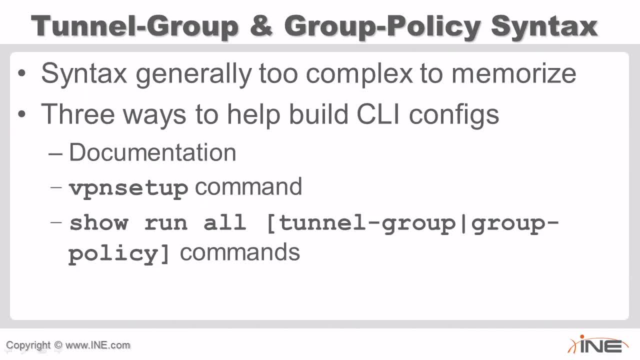 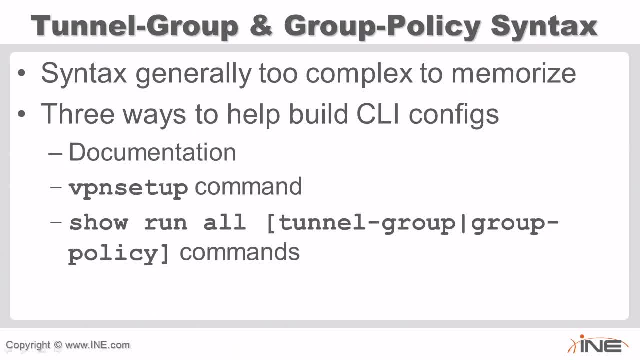 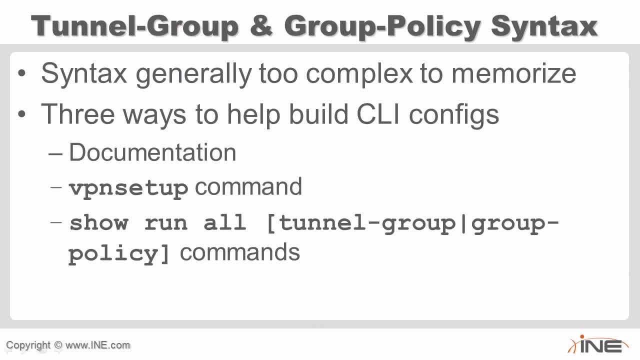 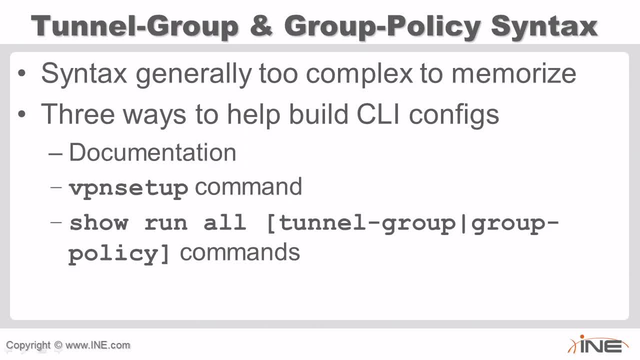 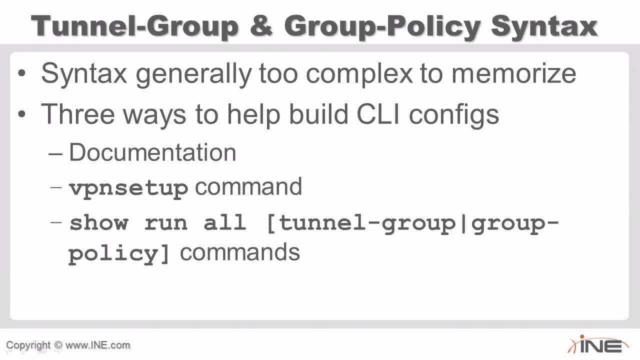 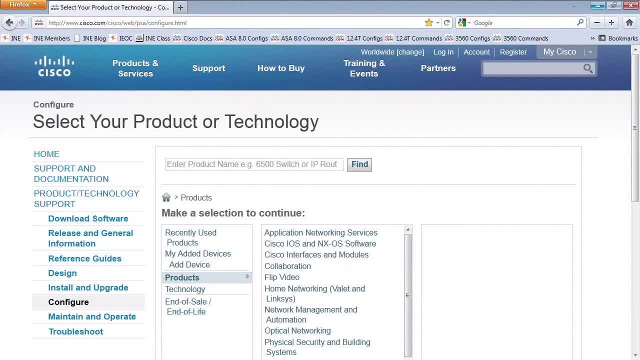 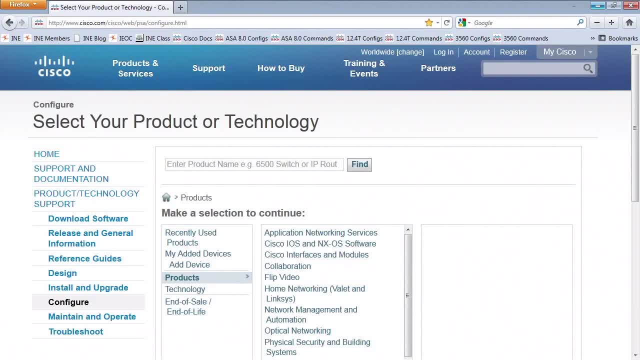 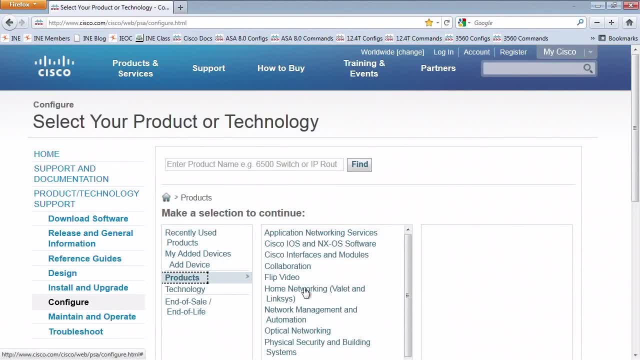 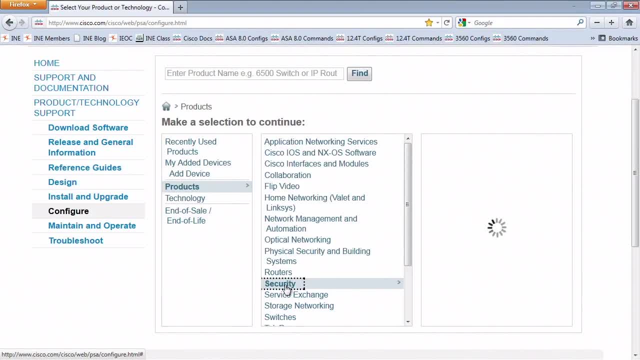 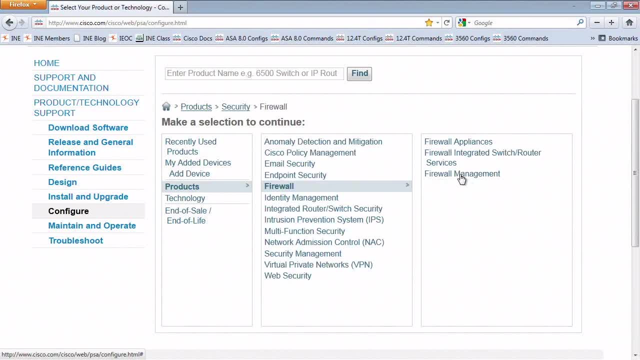 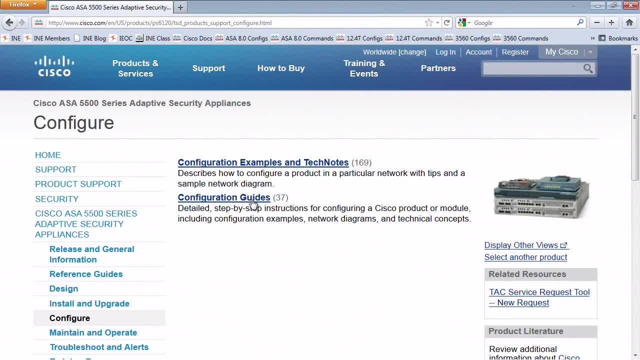 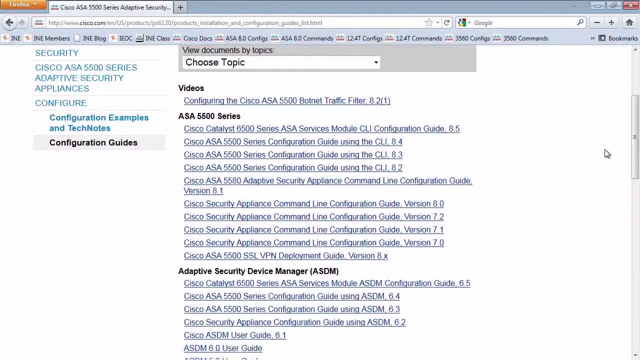 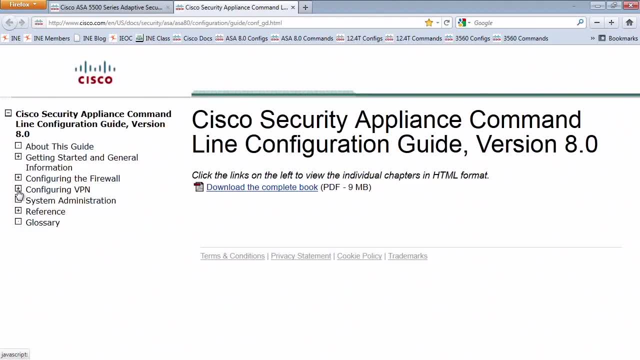 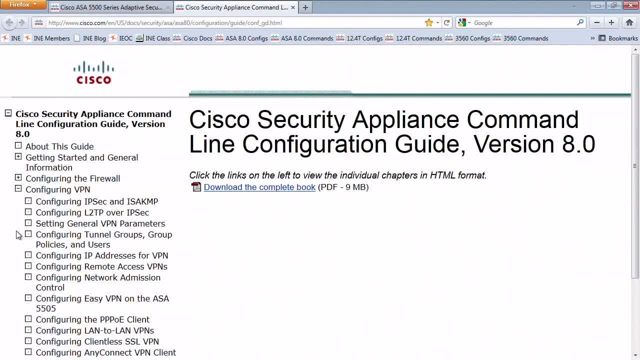 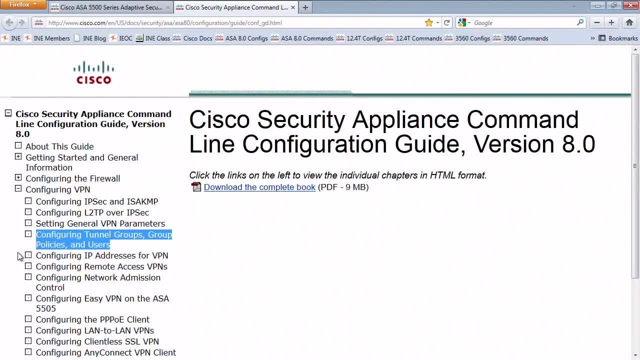 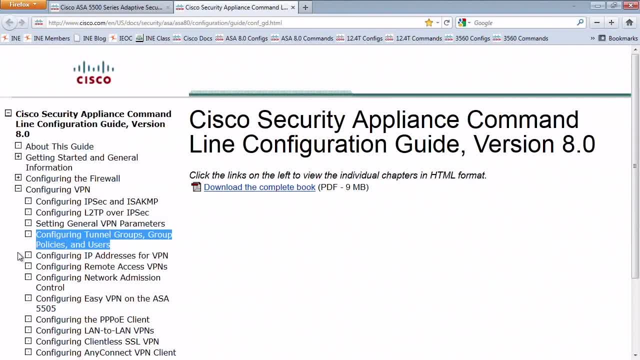 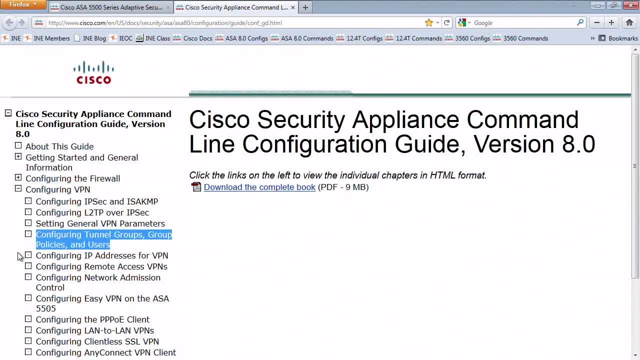 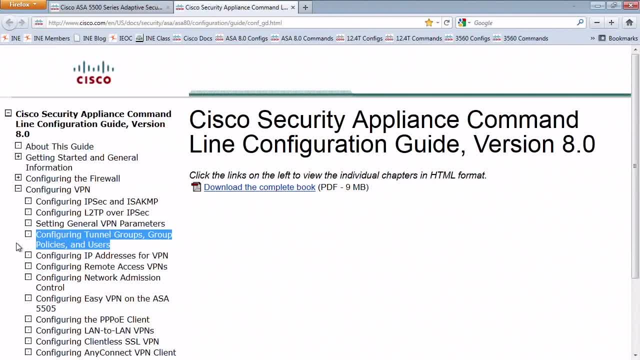 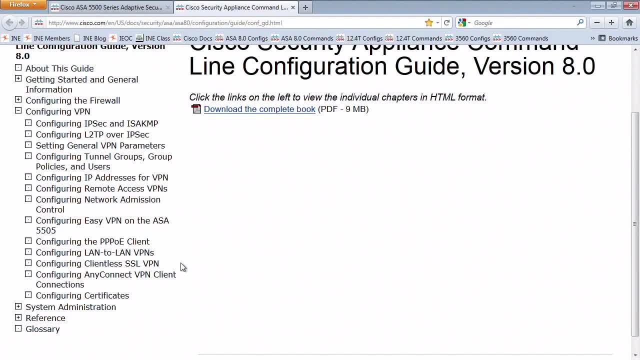 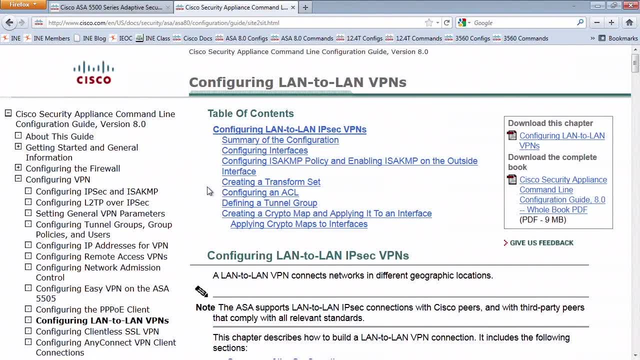 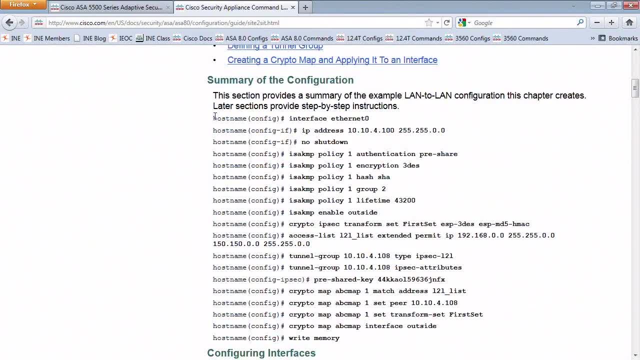 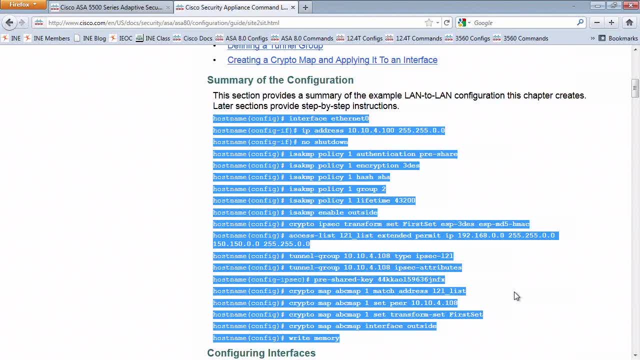 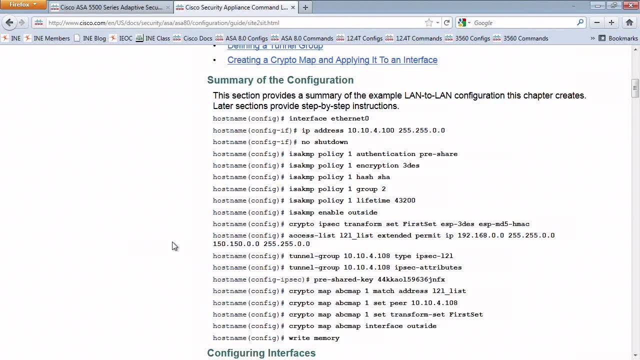 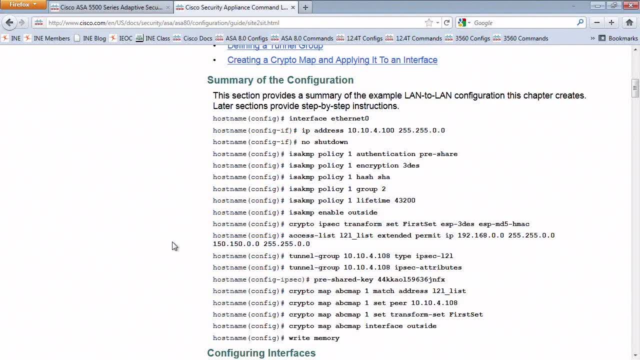 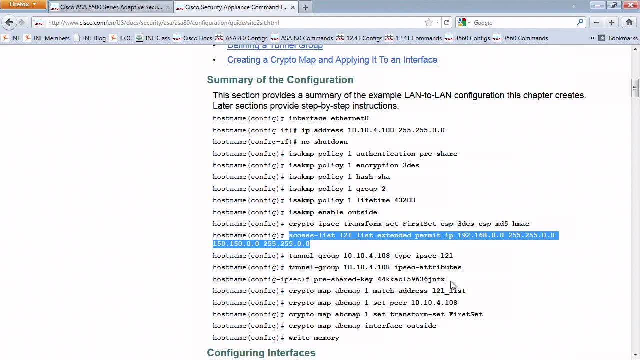 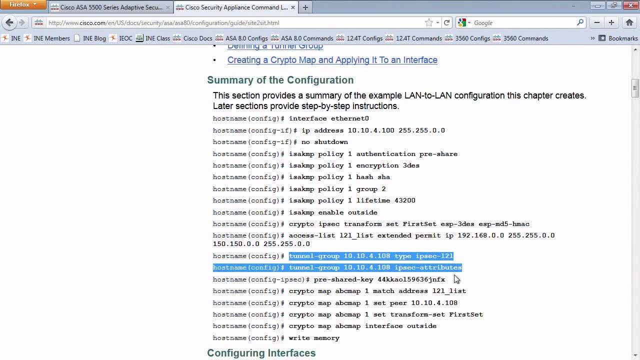 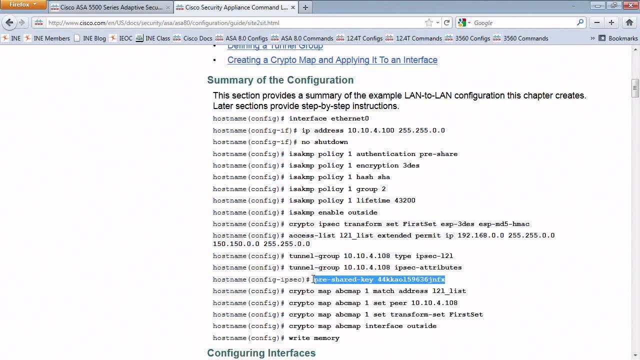 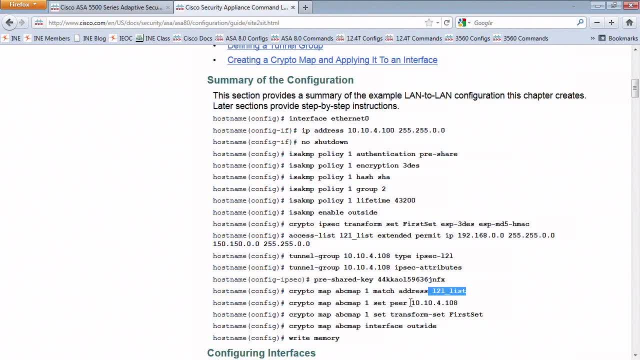 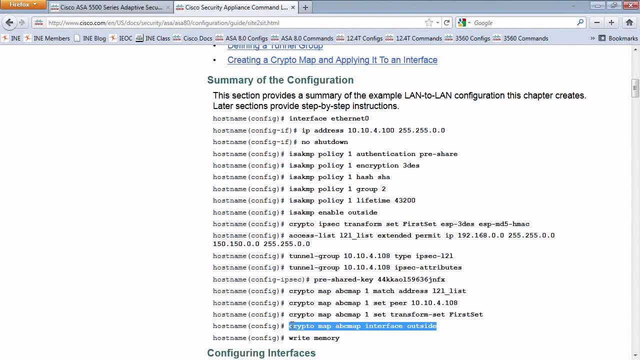 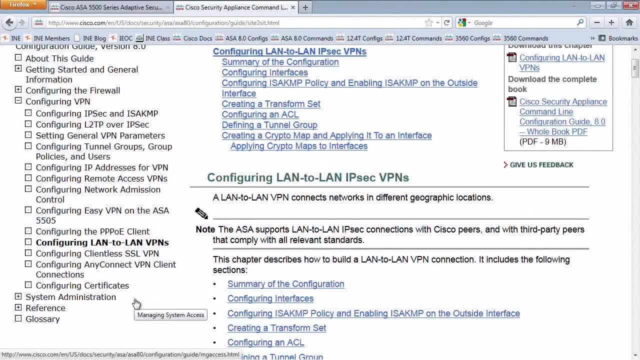 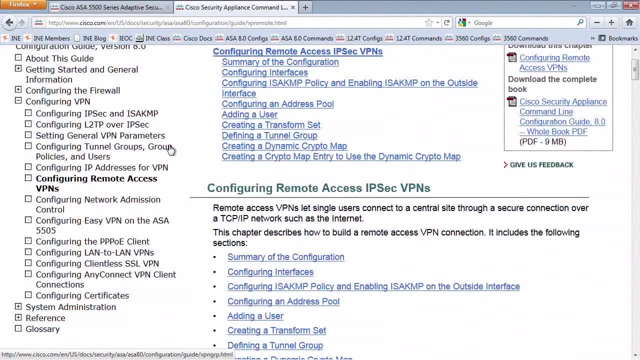 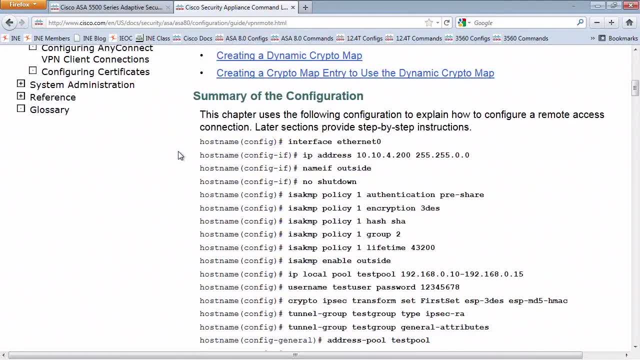 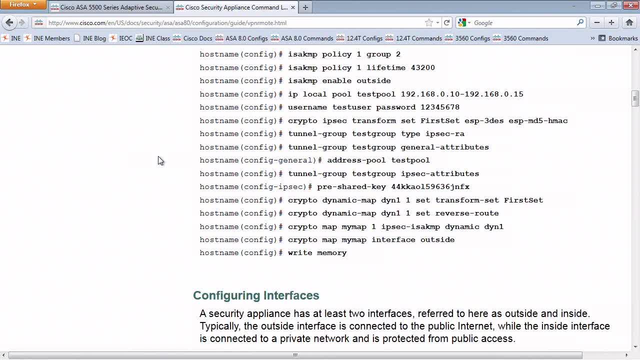 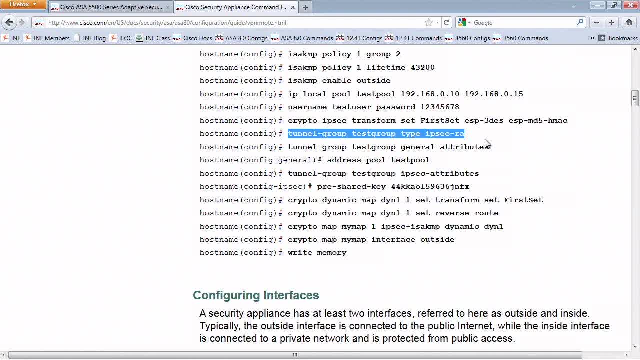 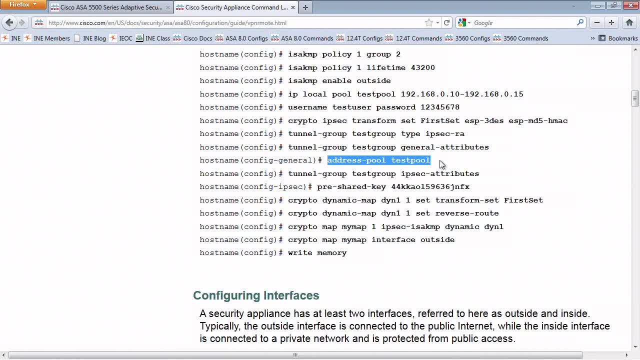 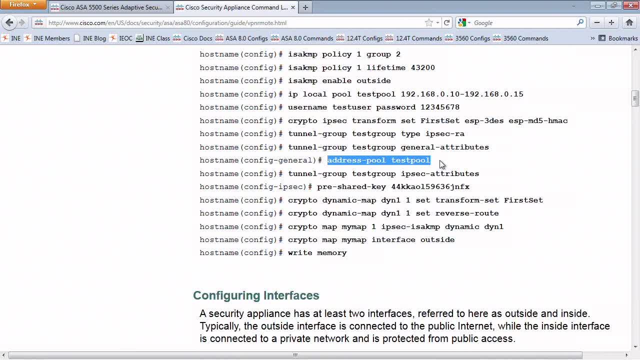 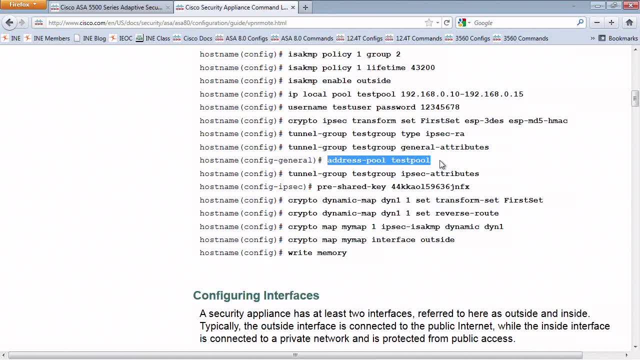 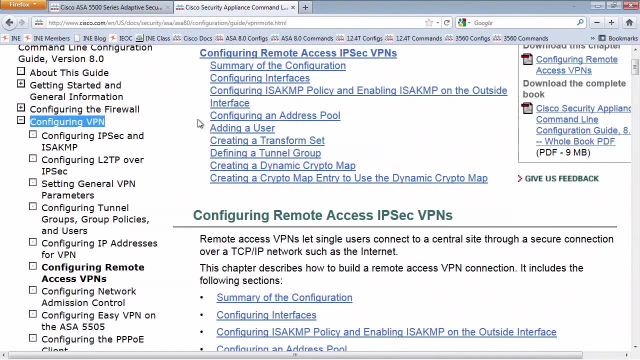 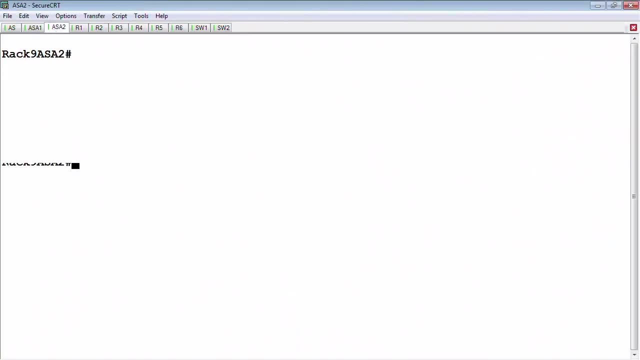 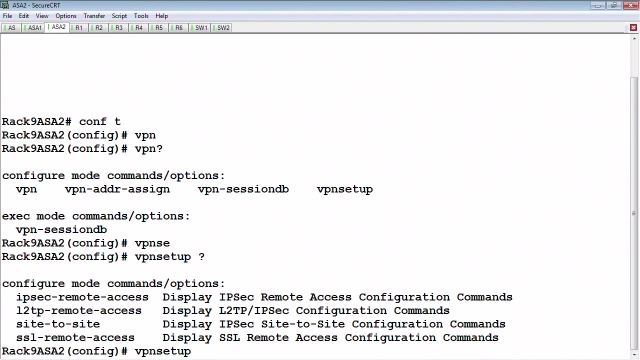 If we were to go to the ASA here and in global configuration, issue the VPN setup command, it says there's four different options. We have either remote access- L2TP remote access, SSL VPN remote access- and then the site-to-site or the LAN-to-LAN VPNs. 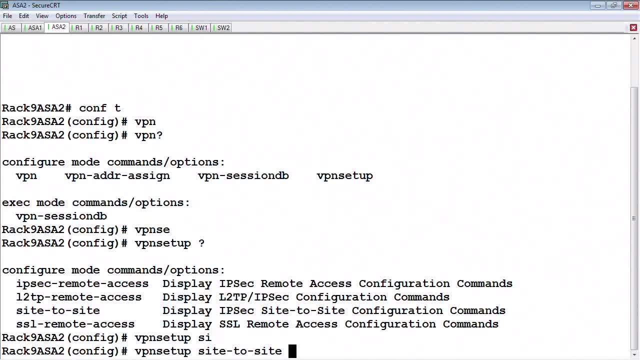 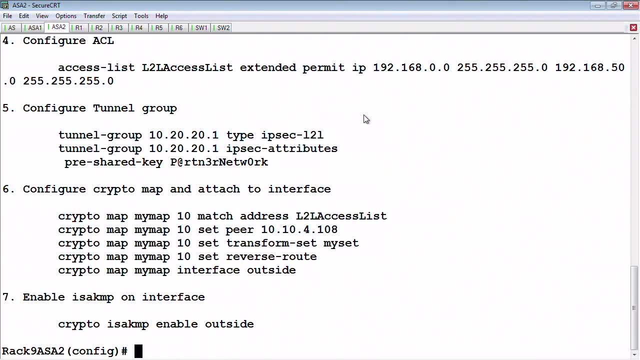 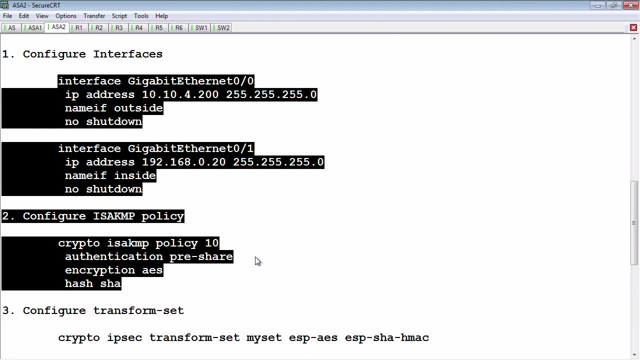 So if we were to say VPN setup site-to-site, and I want to know what are the individual steps that I need to go through, similar to the configuration guide, it's going to show you the final result of the syntax and then you can take this as an example and piece it together in order to match whatever your particular requirements are. 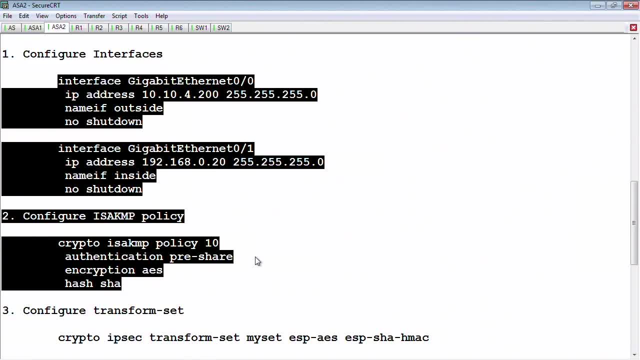 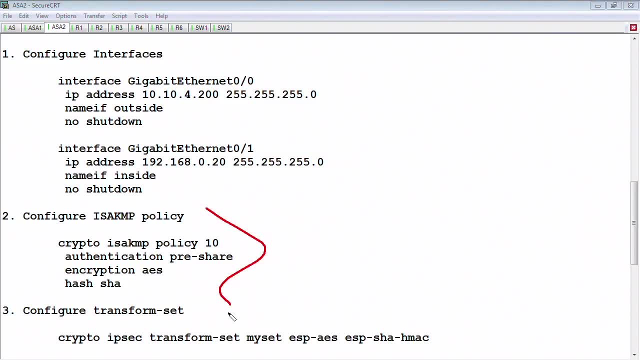 So it's the same logic that we used in the iOS configuration, where first we need to define our phase one policy, That is, things like the authentication, the encryption, the hash, the Diffie-Hellman group and also, if we wanted to define the security association lifetime for phase one. 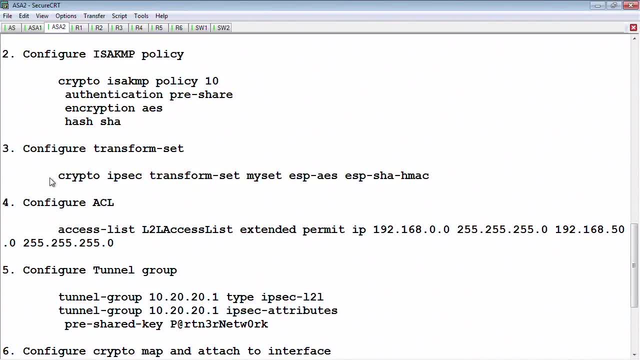 Then we have the phase two transform set, which again is defining how the traffic is going to be treated. The access list is going to say what traffic goes into the tunnel. We have the pre-shared key, which is then referenced from the tunnel group. 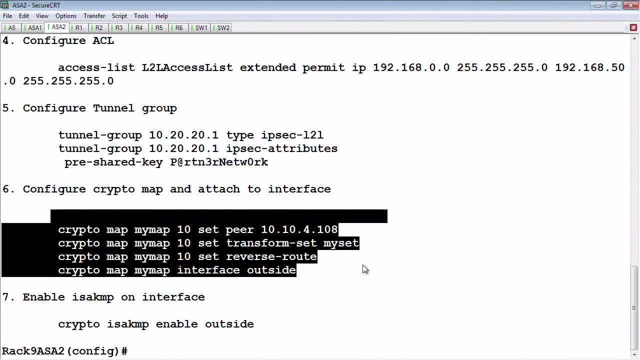 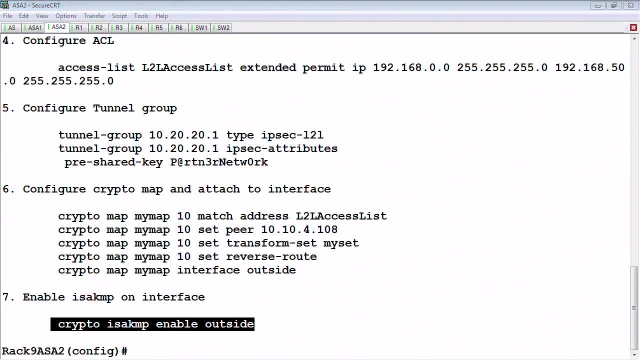 This is tied together from the CryptoMap, CryptoMap is applied on the interface and then, lastly, IsoCamp is enabled on the interface, Where, in the case of iOS, this very last step you don't need to do because IsoCamp is automatically enabled when you bind the CryptoMap to the interface in iOS. 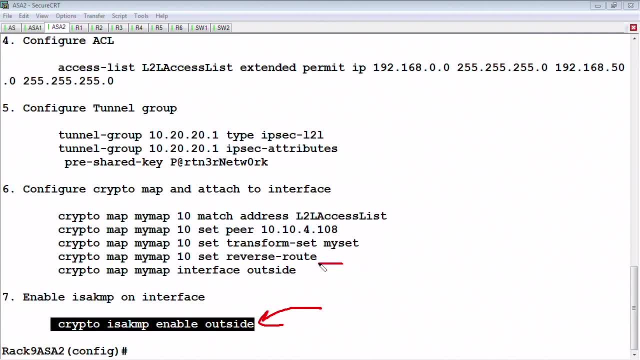 But on the ASA you need to do both of them: You need to assign the CryptoMap to the interface and you also need to define or enable- I should say you need to enable- IsoCamp on that interface as well. Now the last option again is going to be the show run all command, where the documentation does show us the basic example of piecing this together, as does the VPN setup command, but it really doesn't show us all the individual options of what we can do with the CryptoMaps, with the tunnel group and with the group policy. 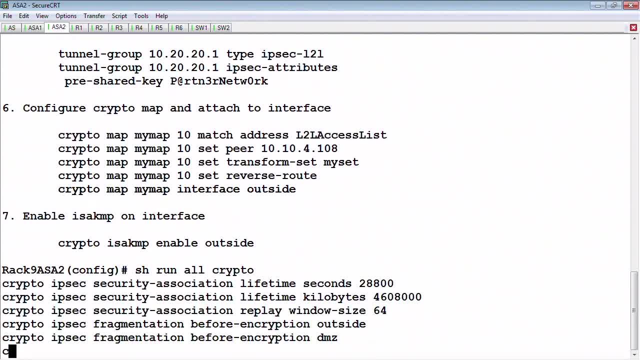 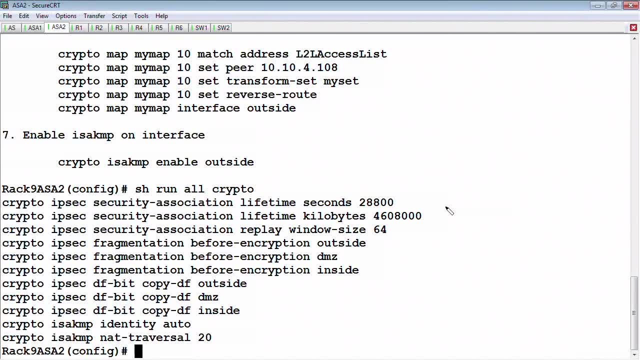 So if we were to look at the show run all crypto. this is going to show us some of the defaults that the ASA has, like what's the The phase two lifetime security association? lifetime values. We have this in a time value in seconds. 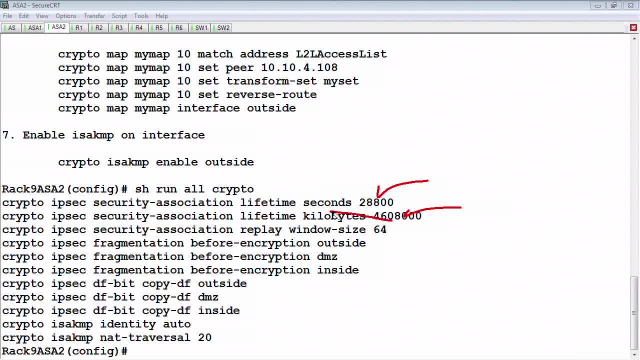 We also have it in kilobytes. The replay window size would control the receiving duplicate packets, which is the anti-replay feature of IPsec. We also have options for fragmentation. It says the don't fragment bit should be copied from whatever the settings are. 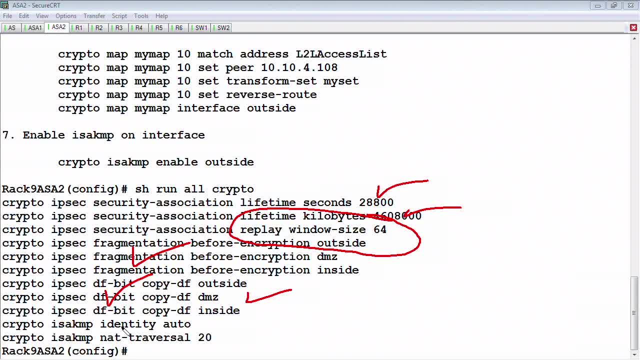 Most particular interfaces And then the IsoCamp NAT traversal feature is on automatically. So we'll come back and look at some examples both with iOS and with the ASA. when the endpoints of the VPN tunnel are behind a network address translation, whether that's going to be a potential issue if we're allowed to tunnel the traffic over UDP or tunnel it over TCP or do a direct one-to-one mapping of ESP. 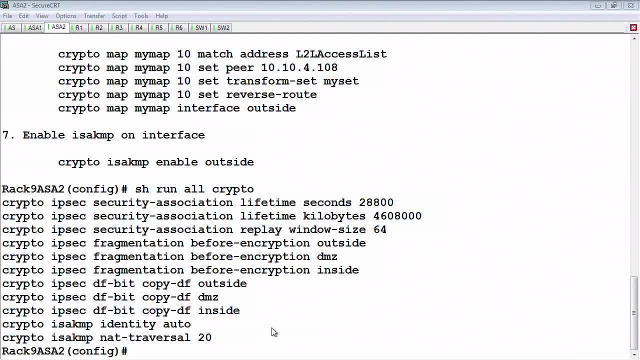 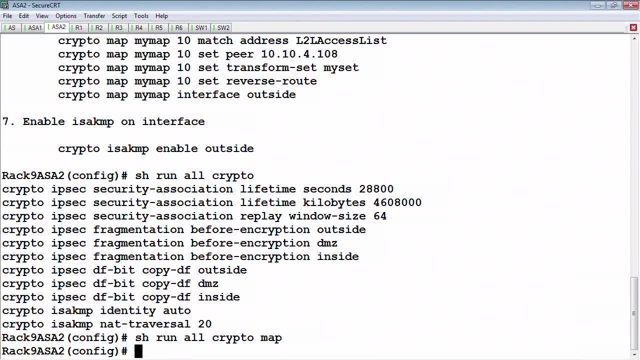 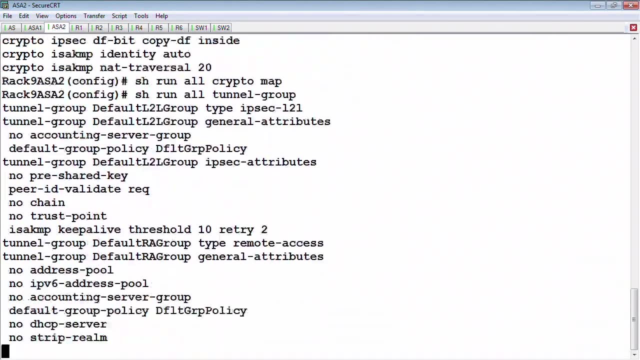 So this one here is going to help us out: the show run all crypto. We could also look at the show run all crypto map, which right now we don't have any crypto maps configured, so it's not going to show anything. But the other two that are useful are the show run all tunnel group, which here we could see. it shows us the default LAN-to-LAN group options. 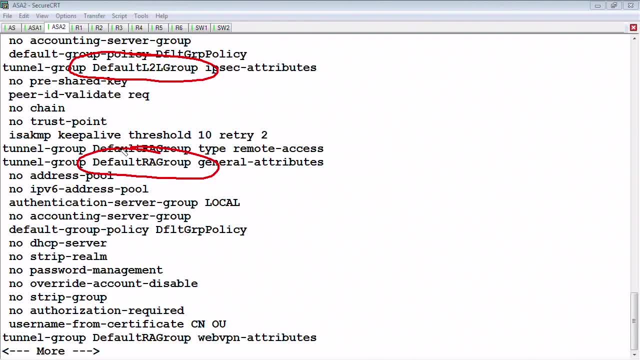 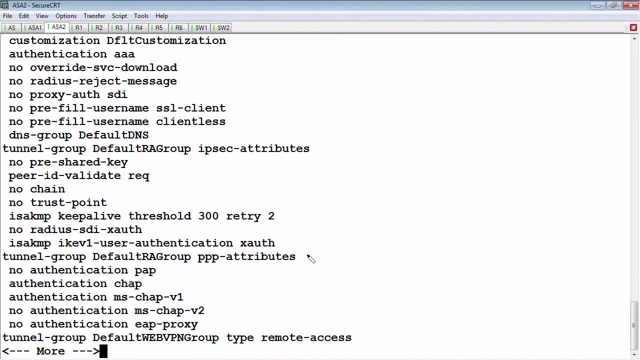 The default remote access group options. Then, Within these individual default groups, there's separate type of sub-attributes, Like we have PPP attributes, IPSec attributes, web VPN attributes. Most of these are going to be for the different remote access groups. For the LAN-to-LAN tunnels. it says that the default group policy or, excuse me, the default LAN-to-LAN group is an IPSec LAN-to-LAN tunnel. It is calling the default group policy, Which has the name of default group policy. 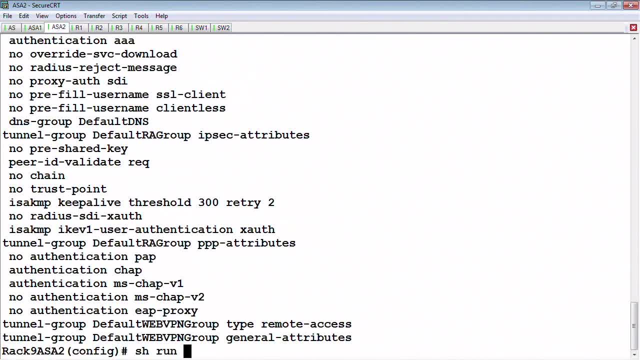 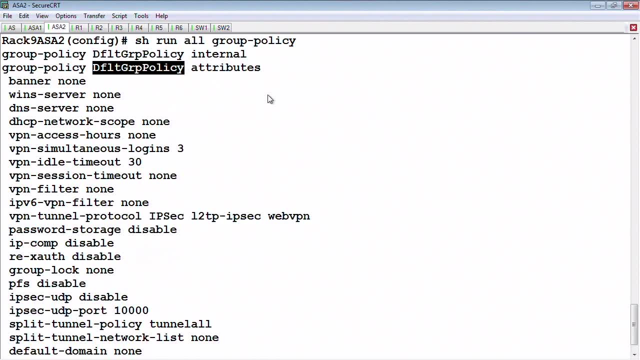 So then, if we were to correlate this with the show run all group-policy, It says we have the default group policy, which is defining things like the message of the day banner. when you connect with your VPN client, What's the win server, the DNS server? 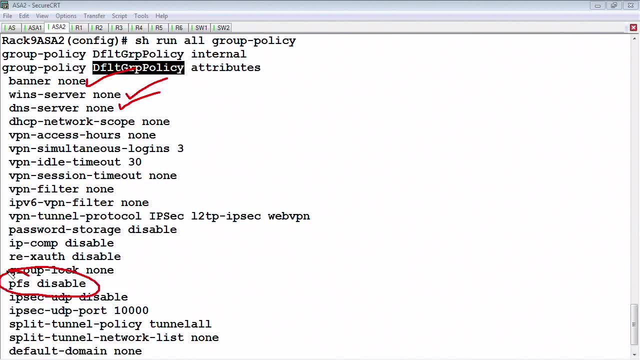 Whether perfect forward secrecy is on or off, Whether transparent tunneling is enabled, Whether transparent tunneling is enabled, What's the split tunneling policy? But you can see a lot of this stuff is self-explanatory, But the problem is that there's so many different pieces of syntax here. 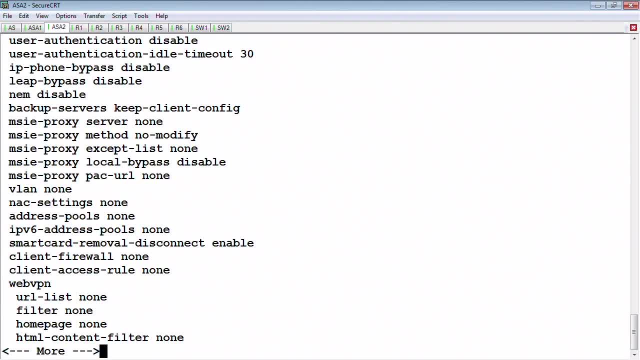 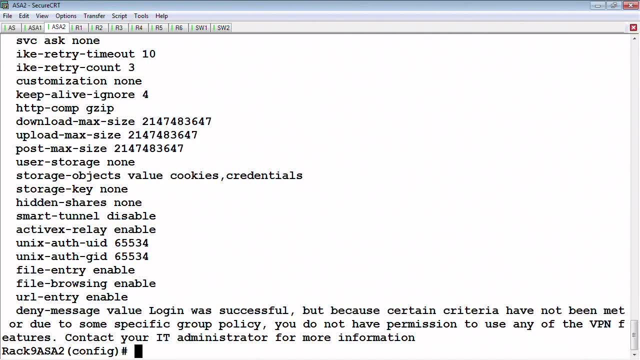 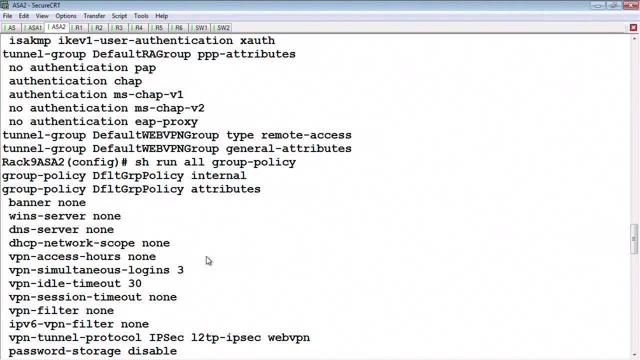 It would be very difficult to try to memorize all of this And even from trying to reference this from the documentation, It might take you quite a bit of time to locate the individual command or the individual option that you're trying to change. So, using this output, the show run all group policy and the show run all tunnel group. 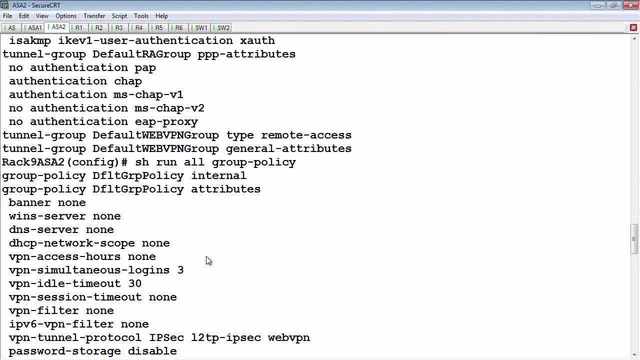 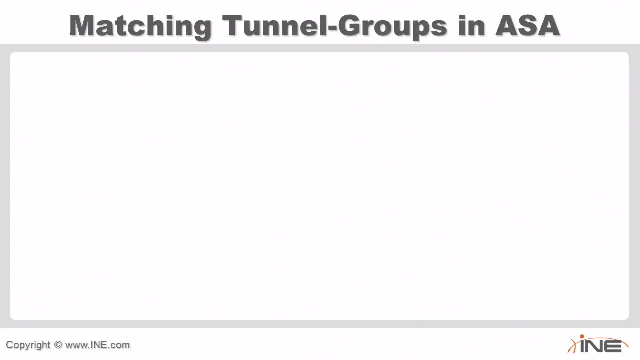 Is going to cut down on the amount of time That you need to piece all of these configurations together. Now, once the tunnel group and the group policy are actually defined, Then we need to determine when we are initiating a tunnel or when we are receiving a tunnel. 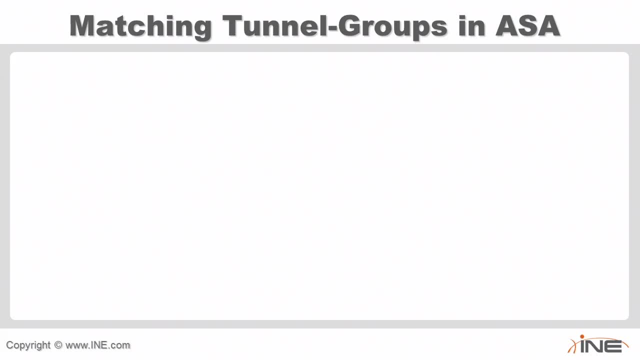 How do we actually know which particular tunnel group that the ASA is supposed to use, And this is going to be based on the name of the tunnel group. Now we'll see. there are cases where we can name the tunnel an IP address. We could give it a string as a name, depending on whether this is going to be a land-to-land or remote access tunnel. 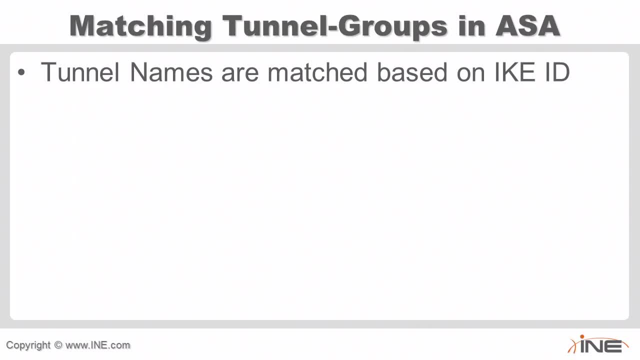 But the tunnel group name is then going to be matched against the IKE identifier Which is exchanged during our phase one isocamp negotiation. So, for example, if we were doing aggressive mode for phase one, Then the tunnel group name is going to be matched against the host name that's in the IKE packet. 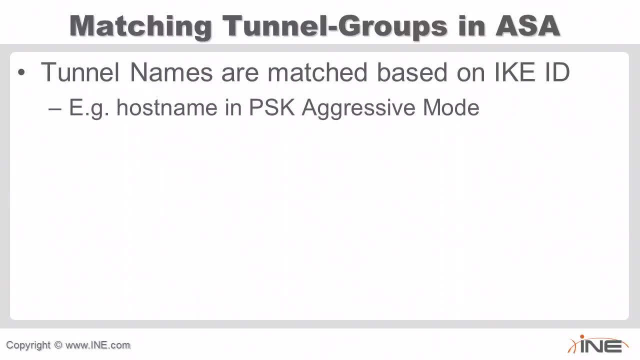 Now, if we were using certificate authority to use RSA signatures or digital signatures, Then we're going to look at the organizational units or the OU field from the common name. So it is going to be significant when we look at the actual signature Or the actual certificate that is issued to a VPN client. 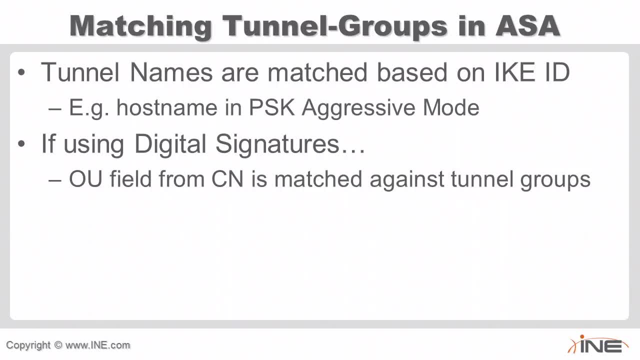 Or is issued to an iOS router or to another ASA. When we're matching this against the tunnel group, We need to make sure that we have the right field In the certificate, matching against our actual tunnel group name. Now we'll also see: in certain cases the IKE identifier may not have a specific string. 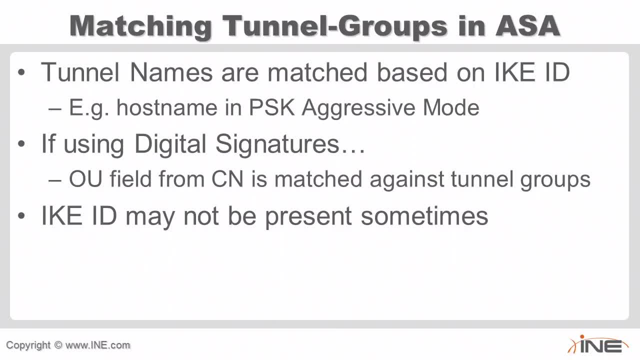 Like the host name or the digital signatures, And mainly this is going to be due to the fact that we are running main mode in phase one. So we talked about the difference between main mode and aggressive mode, Where, in main mode, the identities of the peers are not established. 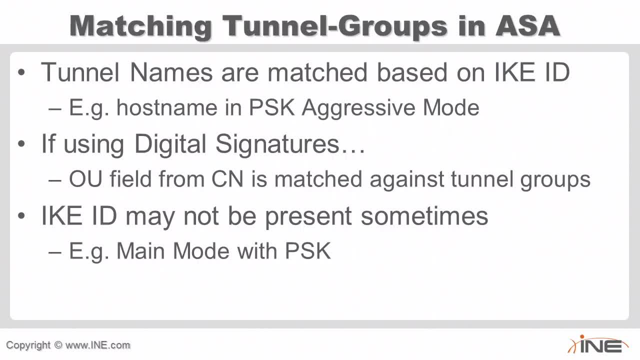 Until the phase one ICCampSA is actually brought up, Whereas in aggressive mode we're sending the IKE proposal Plus, we're sending the identification right at the first step. But the point here is that in main mode, since we don't establish the identities until after the tunnel is up, 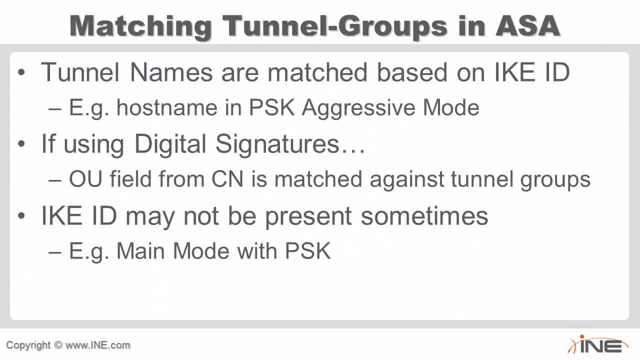 We can't use the IKE identifier to figure out what is the particular tunnel group. And in this case, this is where we are going to use the IP address. So for a basic LAN to LAN connection. So for a basic LAN to LAN configuration. 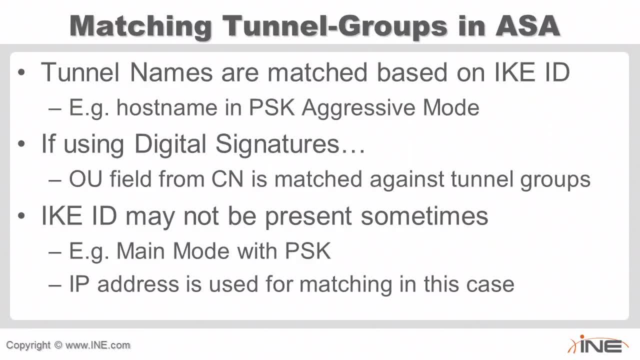 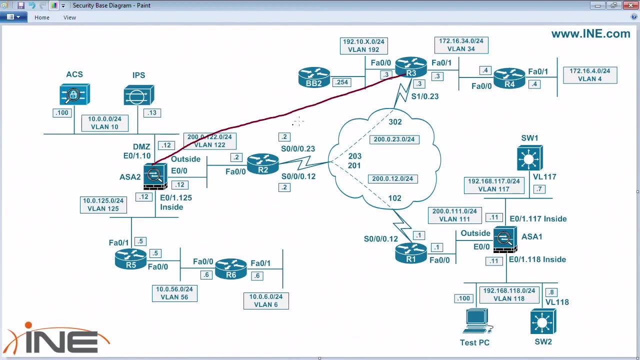 Of ASA to ASA or ASA to IOS. The tunnel group name should match the peer address that we are matching in the crypto map. So we'll take a look at some examples here. where we're configuring a tunnel from ASA2 to Router3.. Where ASA2 is going to say that the tunnel group's name is the address that Router3 is listening for. 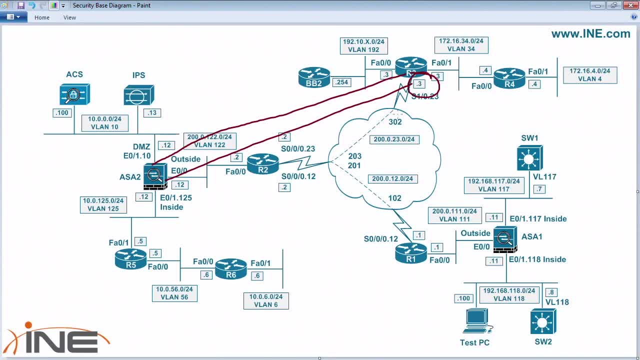 And where Router3 is initiating the tunnel from. If Router3 was sourcing the tunnel from its loopback address, That's what the tunnel group name would be. So, essentially, whatever address that we have set peer as inside of the crypto map, That needs to match what the tunnel group name is. 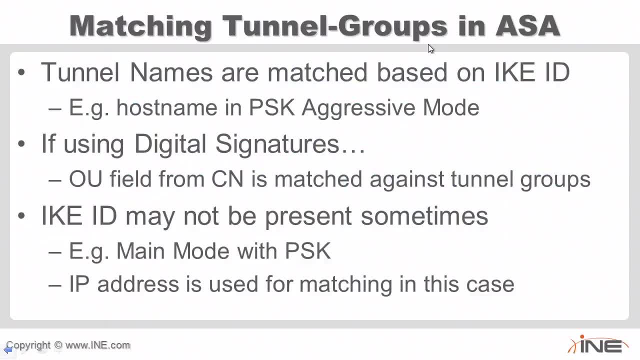 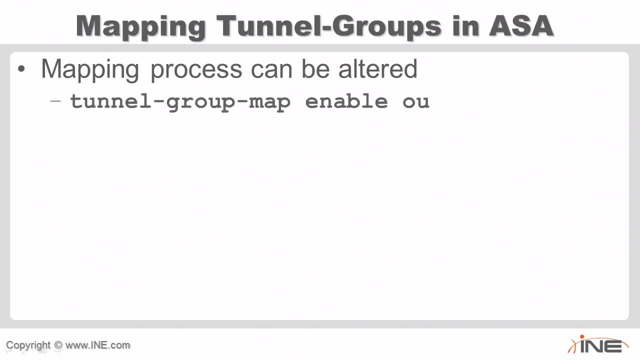 Now the actual mapping process can be changed. There's a couple commands on the ASA that are going to control this, Which are: the tunnel-group-map enable We could use the organizational unit. inside of the digital signature, We could use the IKE identifier. 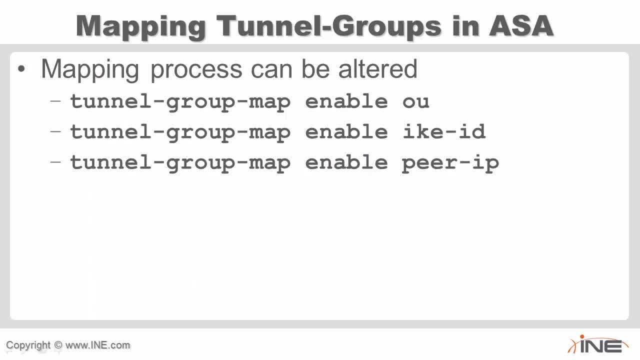 We could use the peer address And by default all three of these are enabled. Now, if, for some reason, we cannot match any of the names, Then we're going to fall back to the default tunnel group, Which is set to the default RA group. 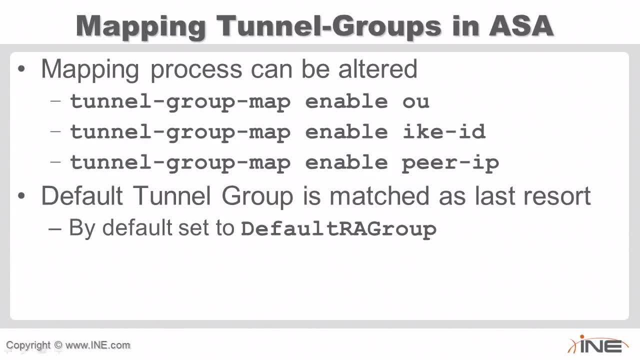 Automatically. So essentially what this means Is that if we were configuring a land-to-land tunnel, But for some reason we could not map the peer address Or the signature for that particular tunnel, It means that it's going to fall back to the default remote access group. 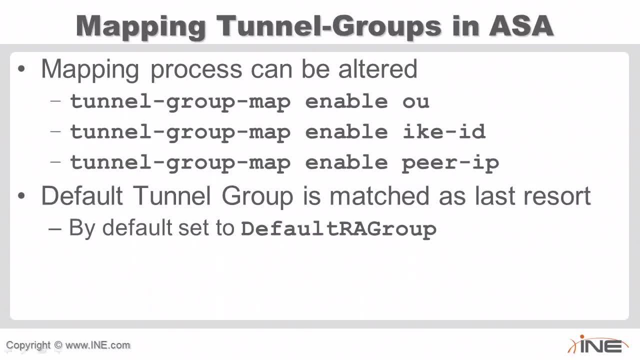 Which is probably not what we're trying to accomplish. So when we look at the configuration here, We'll look at some correct configurations And then some incorrect configurations. Look through the debugs and the show commands To figure out: is the tunnel group properly being mapped? 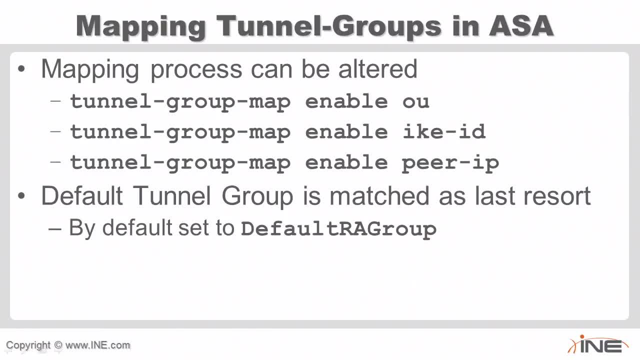 Or is it falling over to an incorrect group Or falling over to the default remote access group? Now you can technically change this. If you say the tunnel group map default group, We could specify the name And you could see these options. if you look at the show, run all tunnel group map command. 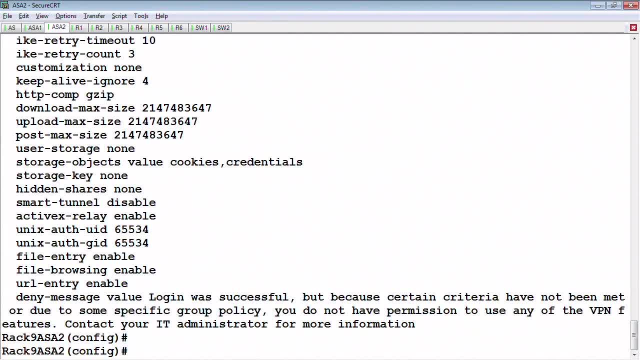 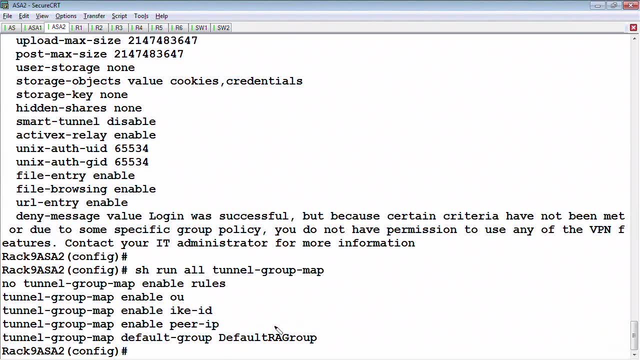 So if we were to look at the command line here And say, show, run all tunnel-group-map, It says that automatically. The default group that you would fall back to as a last resort Is the default RA group And you're going to try to match either based on the organizational unit. 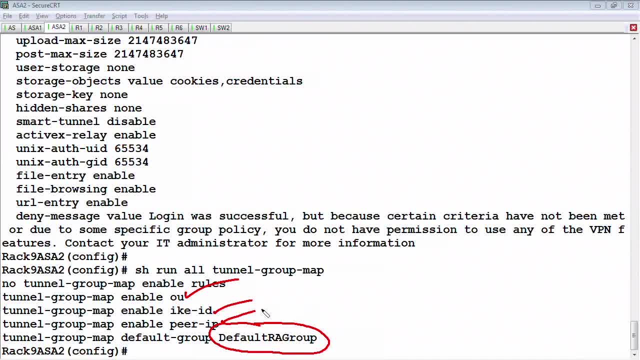 The IKE identifier or the peer address. Then, for advanced configurations with certificates, There's an option where we can configure these tunnel map rules That, based on the particular signature Or certificate that we're trying to use, We can manually map it to a particular tunnel group. 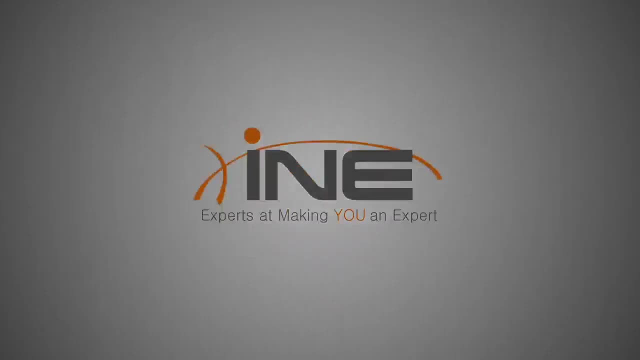 And we can do that by using the default RA group. And that's it. Thank you for watching.